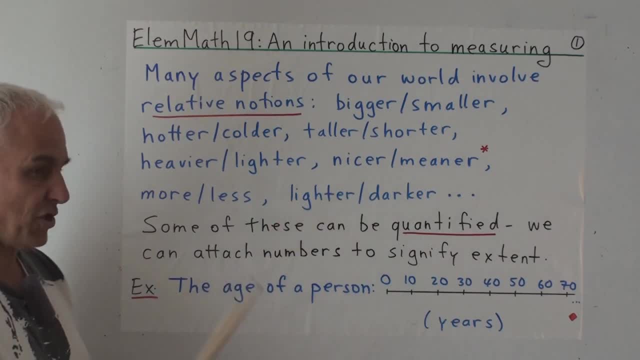 darker. This lighter in the sense of light, while this lighter in the sense of weight. All right, there are quite a few more. So the idea is that what we want to do is we want to look at some of these notions and we're going. 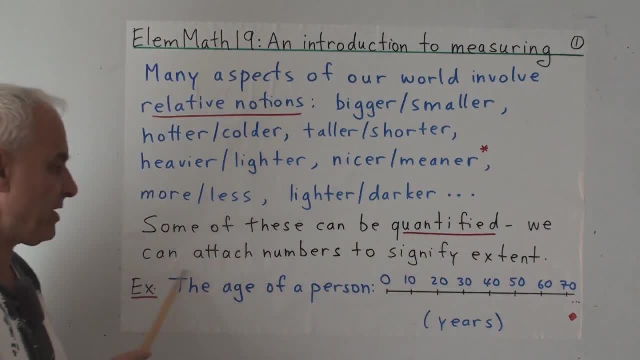 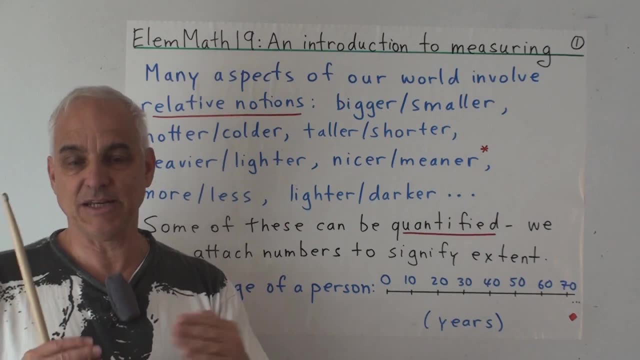 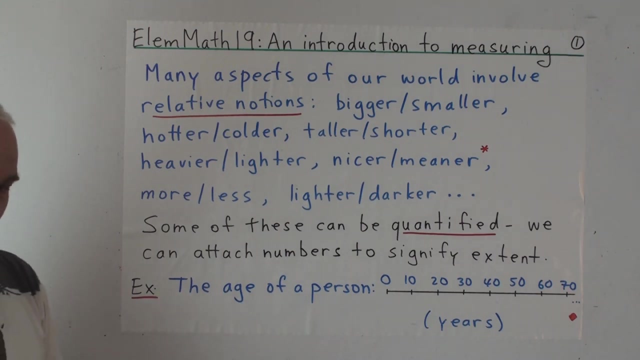 to try to quantify them. That means we're going to try to attach numbers to these qualities to be able to distinguish between different ranges more carefully. So we've seen this already in the previous video where we talked about time in the context of the age of a. 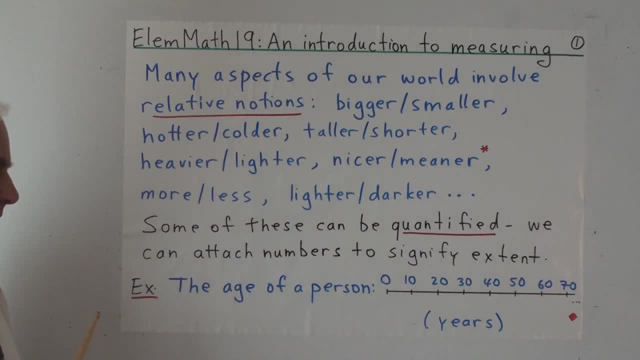 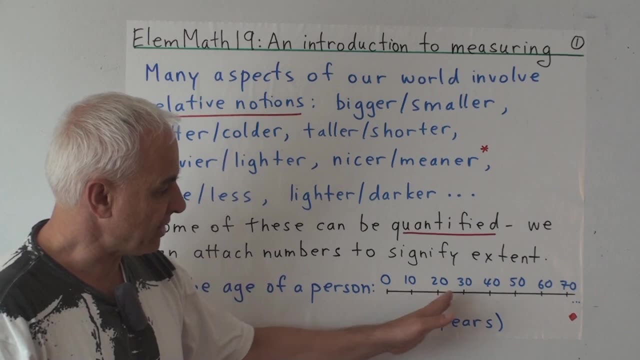 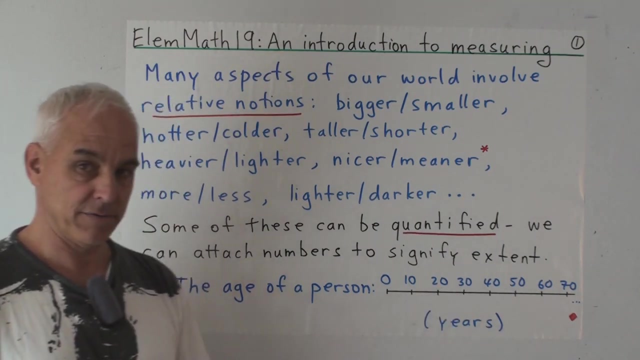 person or the lifespan of a human being, And we introduced the idea of a scale, something like this, where we can plot various years and then position someone on this scale representing how old they are. So if you're 20 years old, you would be represented by that position there. Well, if you're 43. 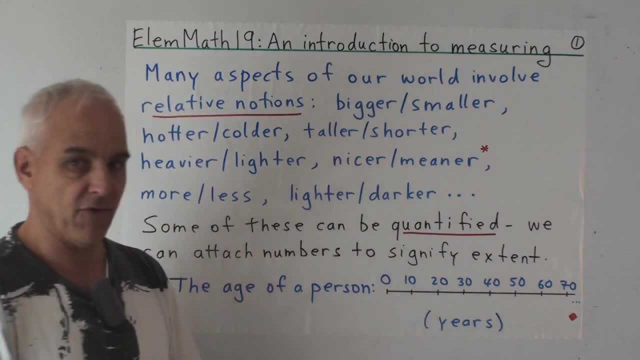 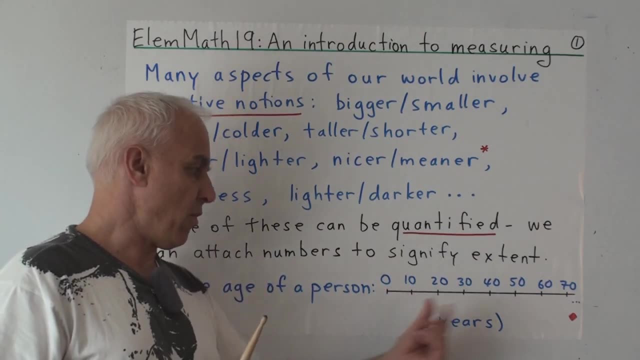 years old, you'd be represented by a position somewhere there, and so on. So this allows us to talk more precisely about things. Instead of saying, well, someone's young, or they're middle-aged or they're old, we can say more precisely: well, they're nine years old. 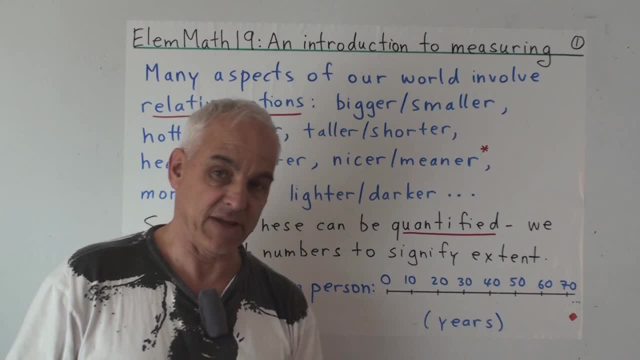 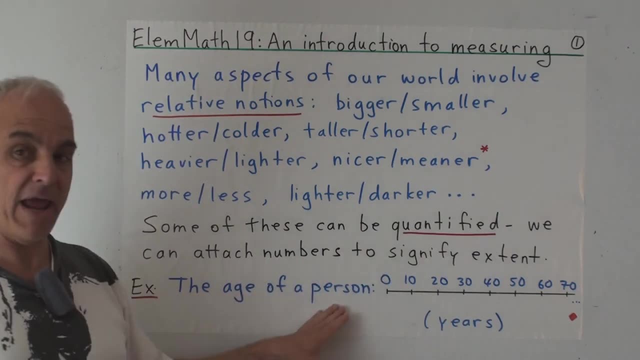 Or they're 42 years old, Or they're 78 years old, And so on. So we want to do that now, not just for time and age, but for some of these other relations. We want to introduce the idea of quantifying things. Now it's not always possible, For example, the distinction 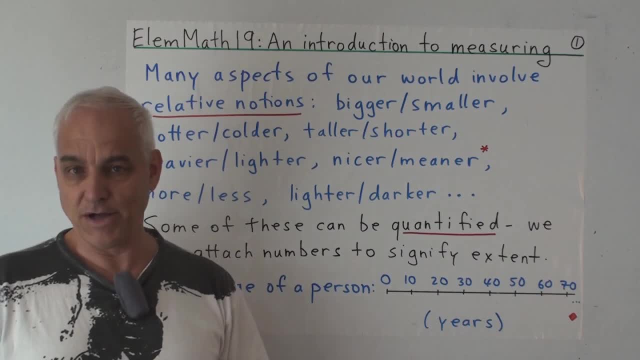 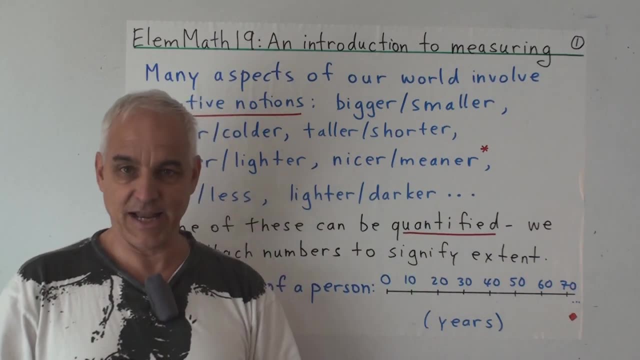 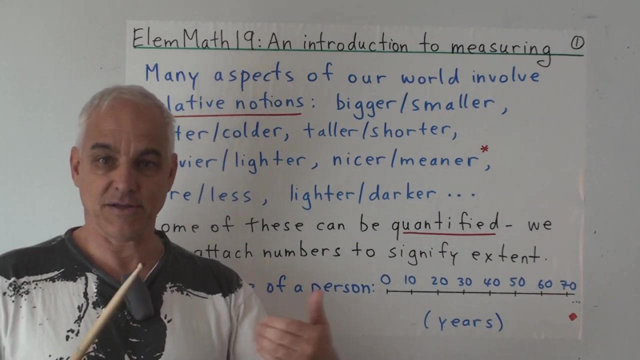 between nicer and meaner is very hard to quantify. You might try, but probably your system of quantifying that will be different from the person next to you. So we're interested in having systems where everybody can agree on the scale that we're introducing. 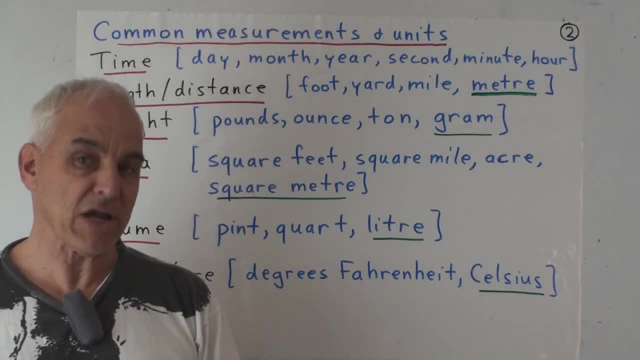 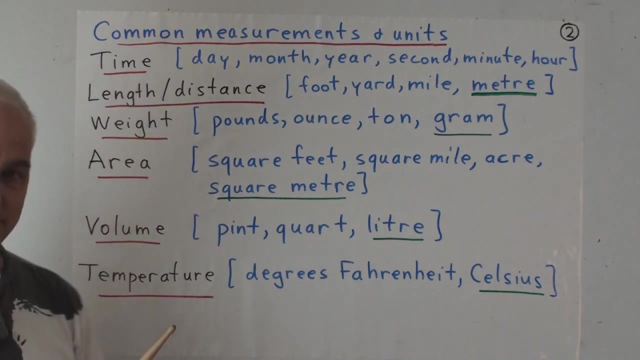 On this slide I've listed some common measurements and the units that they are measured in, So these are quantities that are accessible to quantification. We've already talked about time and we saw that there were quite a few different units that we could use to describe time. We had the day, the month, the year, and we haven't. 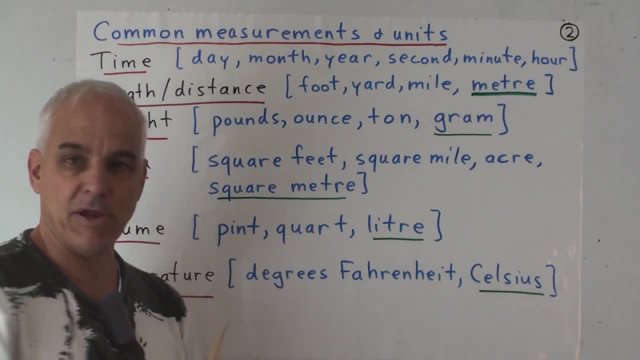 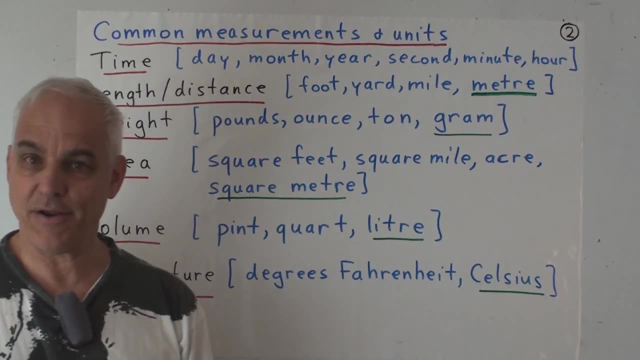 yet talked about the second, the minute or the hour, but they will be familiar to you also. So which of these units we use depends very much on what we're measuring. If we're measuring the amount of time it takes for the Earth to go around the Sun, then we're going to measure. 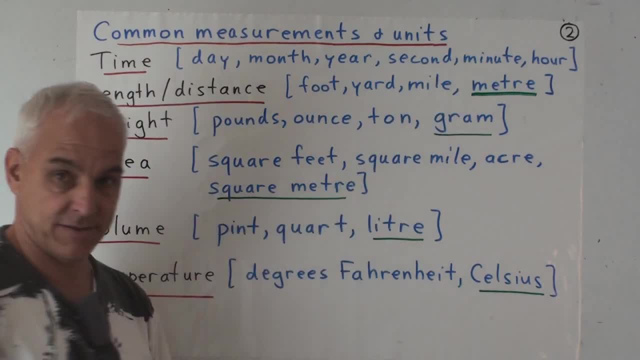 in days, months or years, not in seconds or minutes. If we're measuring how long it takes to run 100 meters, then we're going to talk about seconds, not months or years. So that's a general principle that applies to these other things too. Typically, we have 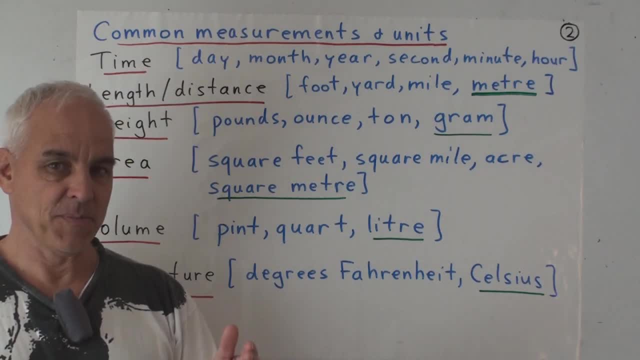 a number of different units and the choice of unit is determined by what exactly we're measuring. So let me introduce one, two, three, four, five other quantities that are very common, that are measurement kind of quantities that we can assign numbers to. The first and probably the simplest one is: 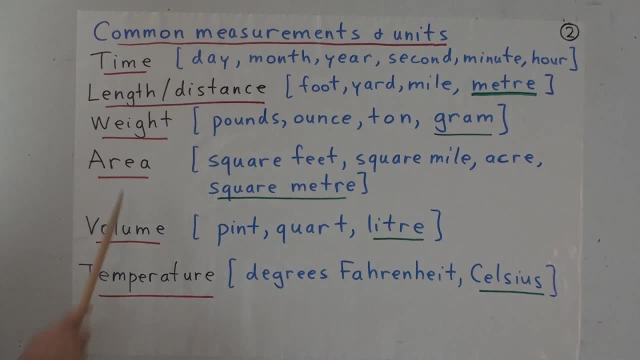 length or distance, and then weight, area, volume and temperature. Now, when you learn a little bit more science, you find out that there are quite a few other things that we can measure, but these are kind of primary ones that are particularly 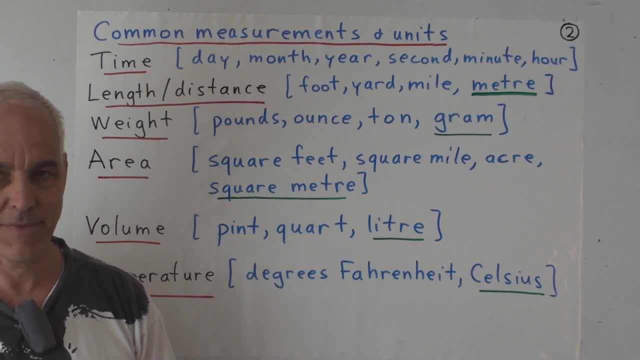 important for children in the years K-6.. So let's have a look at them. The first one: length and distance. Now there's the natural question of: well, what kind of units are we going to measure these things in? And since this is such 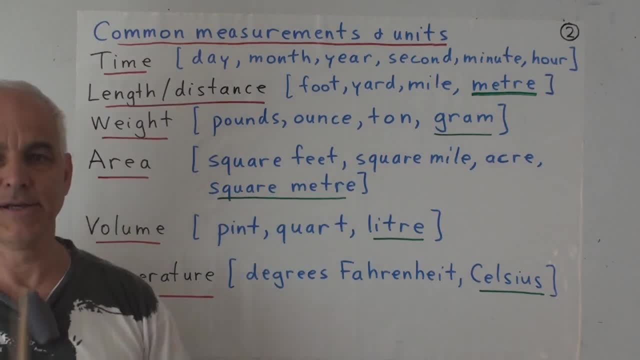 a common and important type of measurement. there is a wide variety of different units available. Some of them, and only a few of them, are the foot, the yard, the mile and the meter. I've underlined the meter here in green because this is a metrical system. 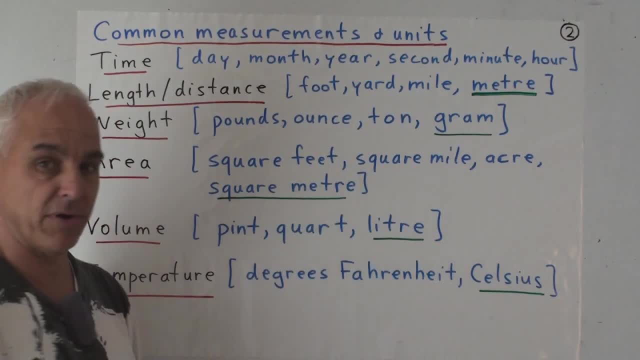 unit, while these ones here are so-called imperial system, and we'll talk about the difference in a little while. There are many others. For example, there's an inch and there's a centimeter and there's a kilometer, and 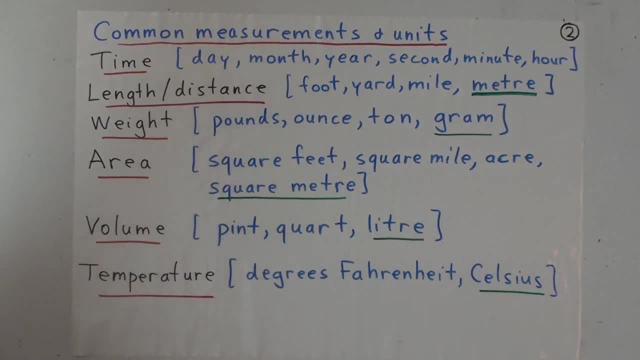 there's leagues and chains and many other things. Okay, when it comes to weight, we're talking about how heavy something is, how hard it is to pick it up, And there we generally measure things in pounds, ounces or tons. 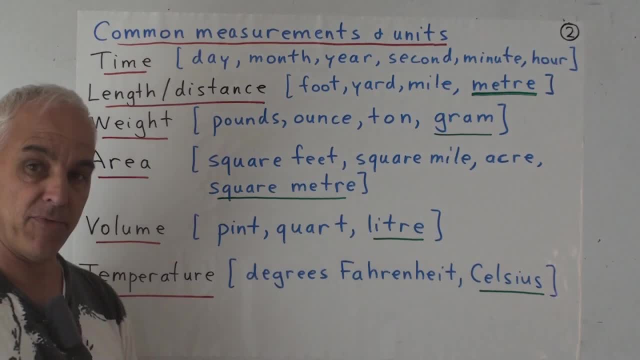 in the imperial system and grams or kilograms in the metric system. Now, while we're talking about the two-dimensional region, the measurement of that is a sort of a two-dimensional version of a measurement of length or distance. So we talk about square. 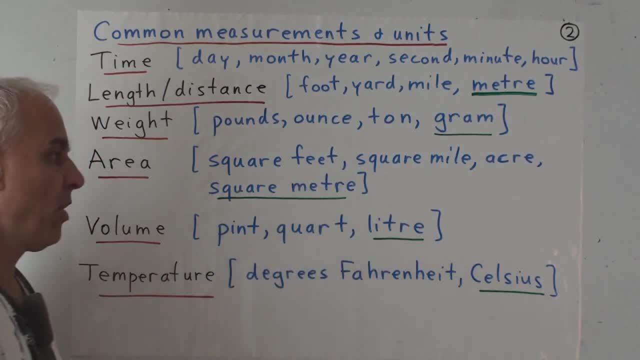 feet or square miles or square meters, and there's a few other ones that are introduced, For example an acre. In terms of volume, we're talking often about a liquid, how much room a liquid takes. For example, about five tons, For example about twenty tons. So this is how many tons aому? 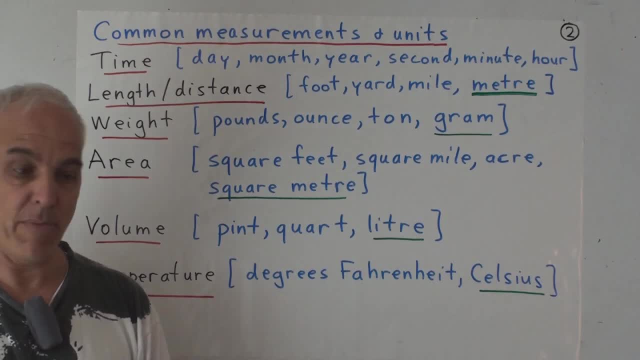 bottle of milk or a gallon of gasoline, or maybe the amount of water in a bathtub or swimming pool. that's a volume question. and again, the units that we choose there. well, there's pints, there's quartz, in the imperial system and in the metric system, the liter, a sort of a different kind of quantity. that's also. 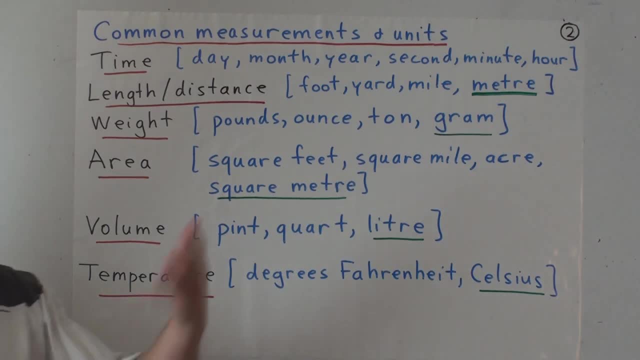 quite important for young people is temperature: how hot and cold it is. so instead of saying, well, it's kind of hot today and or it's cold today or it's, so it's kind of room temperature, we can quantify that by creating a scale, and there are two important scales I used around the world today: the degrees. 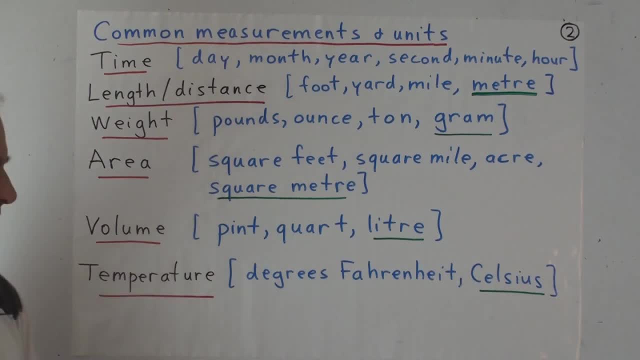 Fahrenheit and degrees Celsius. Celsius, usually more associated with the metric system, perhaps all right. so there's a lot to learn here: that we have to appreciate these various quantities, we have to become familiar with the scales, we have to learn about the units and we have to be able to have some. 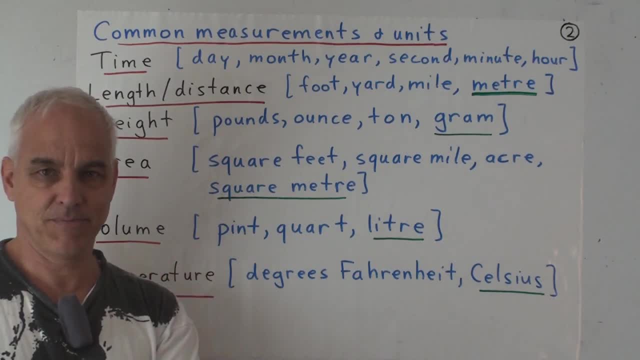 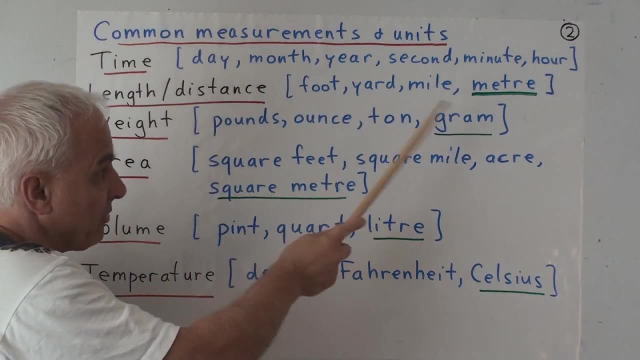 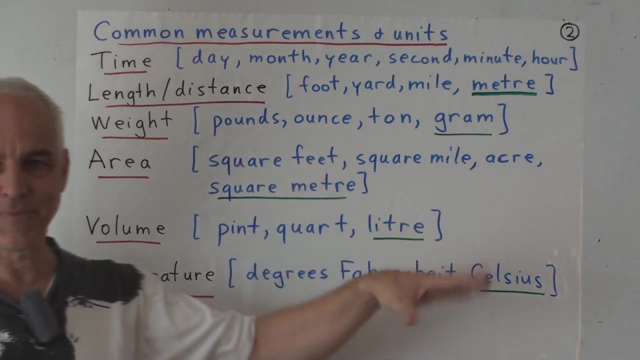 appreciation of the relationship between the units, with the relationship between a day and a month, between a month and a year, between a foot and a yard, or maybe between a yard and a mile, or mile and a meter, and so on and so forth. so there's a quite a lot of learning that has to be done for young people in this general 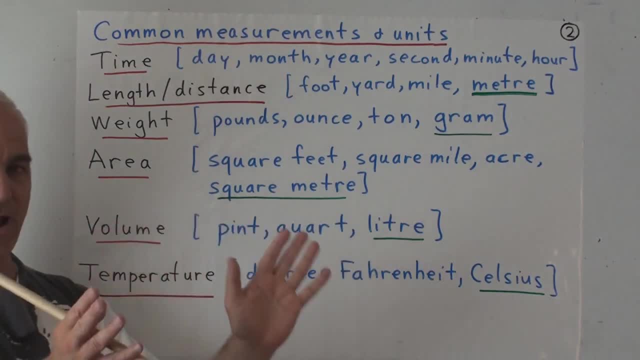 area. just an introduction, This is just sort of laying out a broad direction. Okay, so eventually in the years K to 6, the child should learn what all these words mean and they should end up having a pretty good sense of the physical meaning of. 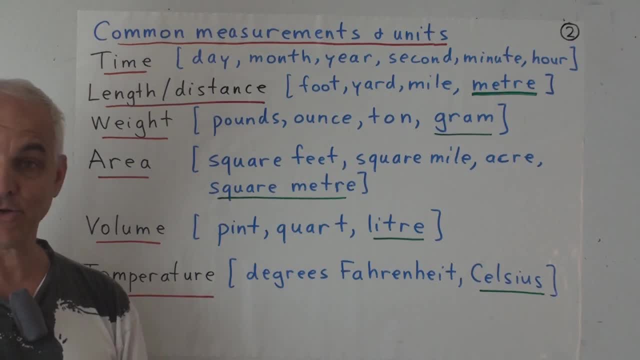 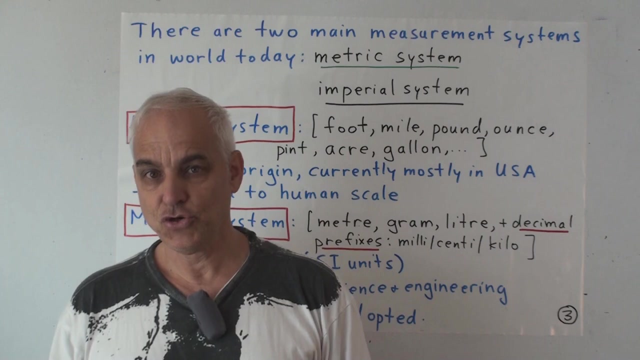 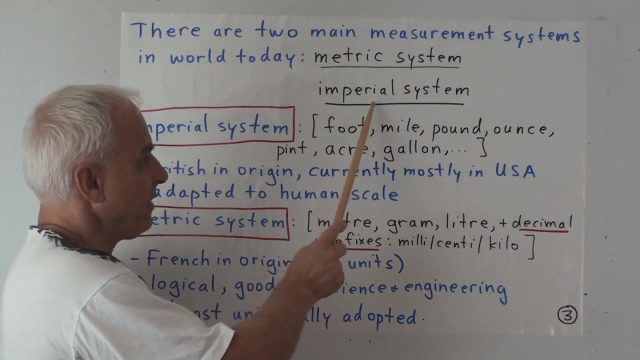 these various quantities and have some experience in actually measuring them. Alright, so today we're gonna stick with the first one. We'll talk about length and distance. As we saw in our previous slide, there are two main systems of measurement in the world today. They are the metric system and the 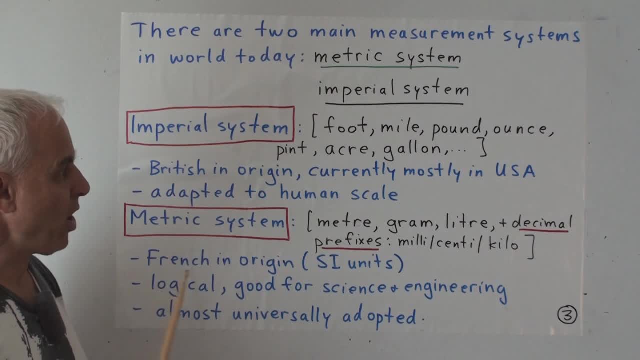 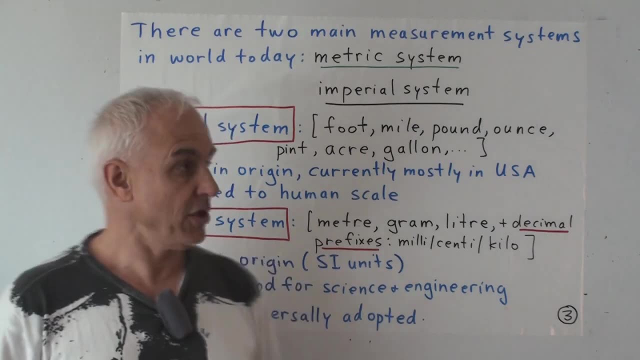 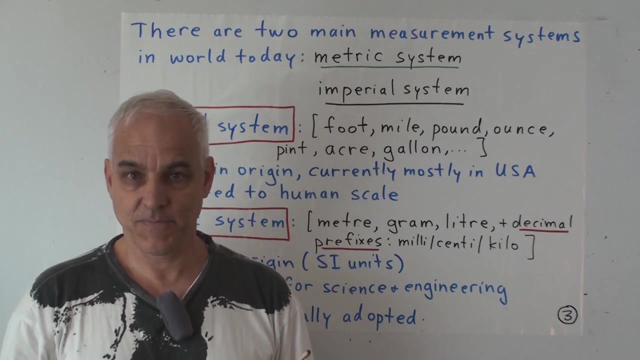 imperial system and which one you use depends almost entirely on which country you belong. Most countries in the world today use the metric system, but there are a few that still use the imperial system, primarily the United States. 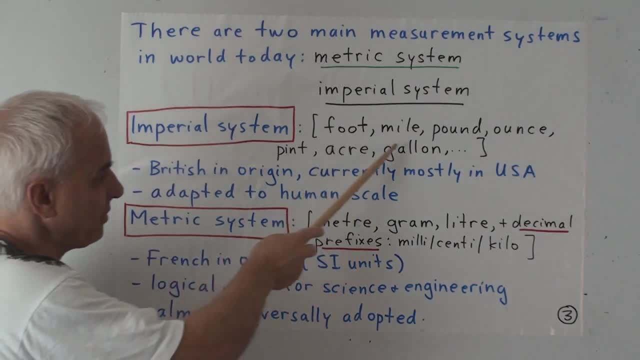 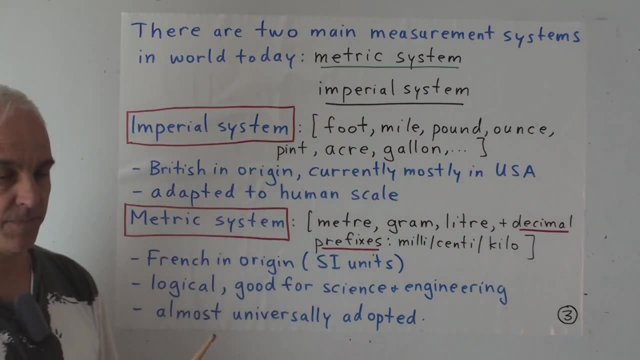 The imperial system, which uses units like foot, mile, pound, ounce, pint, acre, gallon and many others, is British in origin and today it's still somewhat used in Britain, although Britain has moved officially to the metrical system. It's also somewhat used in Canada, although, again, 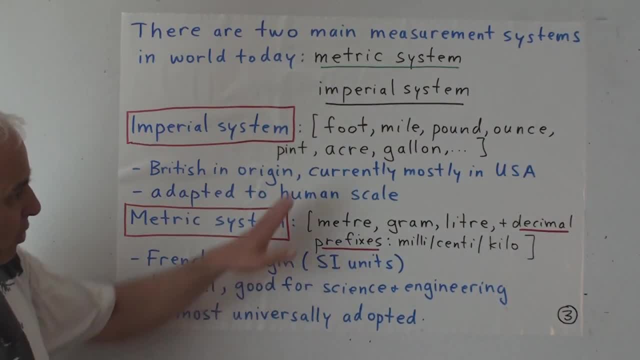 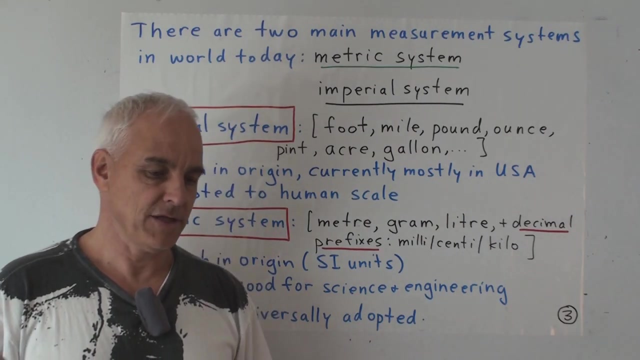 Canada is also in the metrical system. The origins are rather personal. So a foot which is a unit of length around this big was probably, you know, the size of a British monarch's boot, And so it has its origin in human usage. 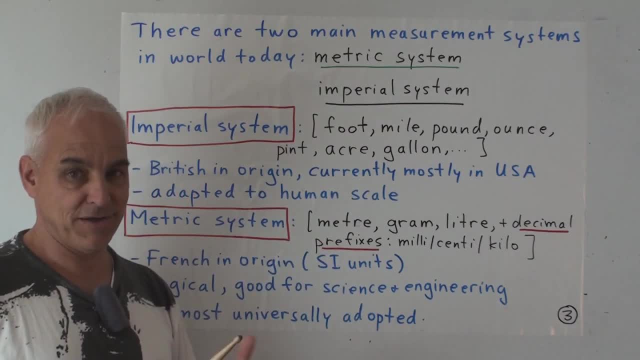 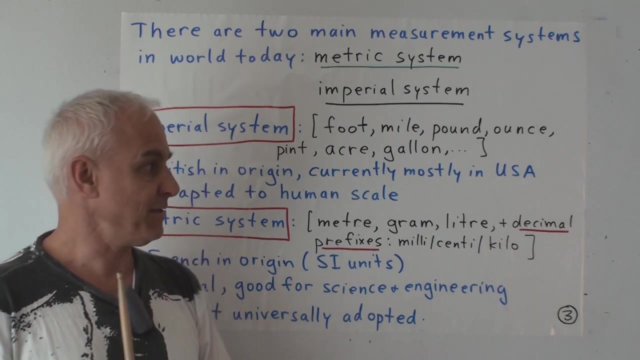 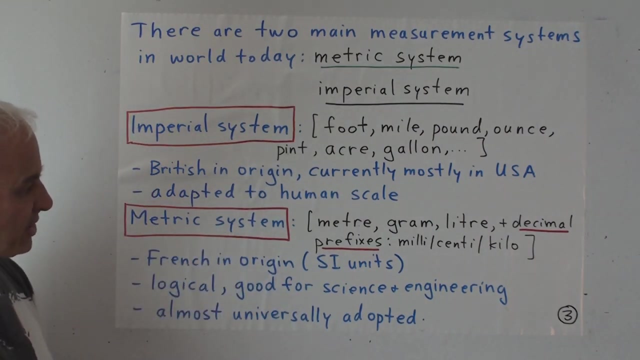 And there's a rather arbitrary aspect between the different units and it takes some getting used to the different relations and certainly complicates the arithmetic of the system the fact that the units relations are rather ad hoc and hard to remember The metric system, which uses units like the meter. 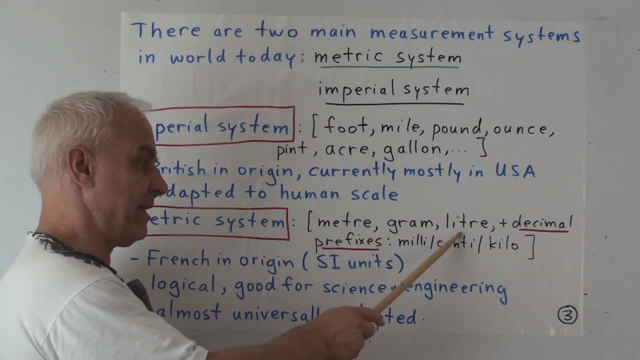 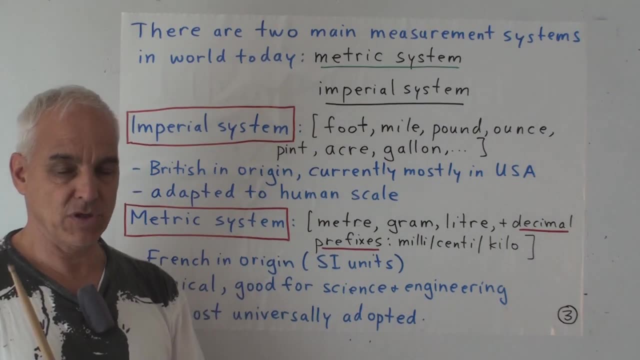 gram litre. meter for length, gram for weight, litre for volume, then organizes itself using a decimal system, So it's much more logical and systematic. So once you've defined a meter for length and meters for length for length, which is about this big, Then other units of length are either: 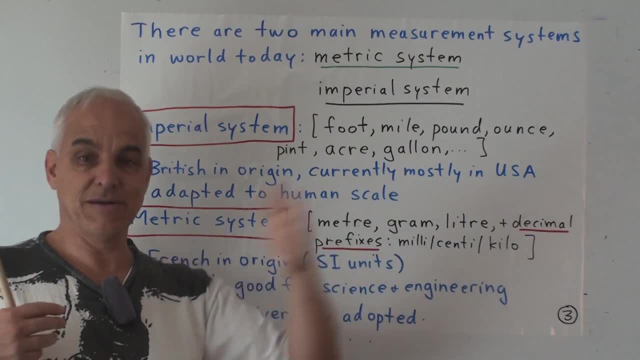 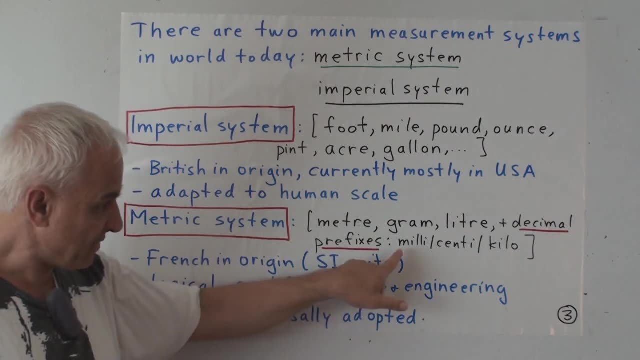 multiples of 10 from the meter, or divisions of the meter into 10.. So we always multiply by 10 or divide by 10.. And then there are these various prefixes that go in front of the word to tell us how many multiples of 10 we're. 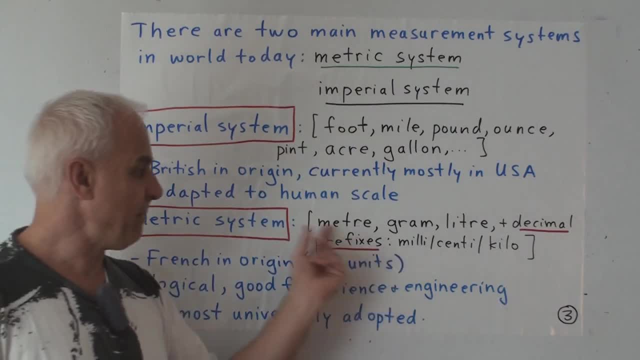 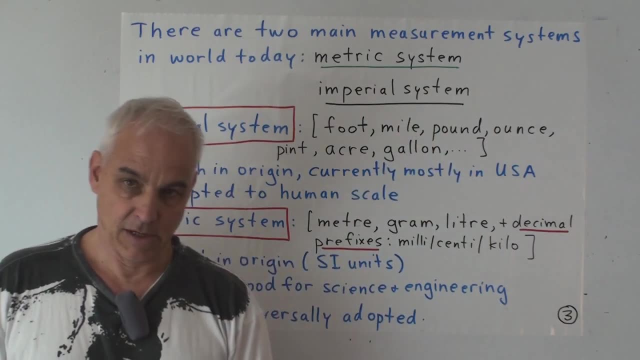 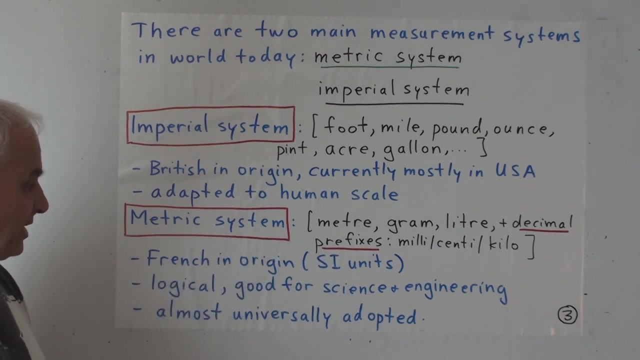 dividing by or multiplying by. So a millimeter is very small, like this a centimeter, or something like this: A kilometer? well, that's two-thirds of a mile roughly. So this is French in origin. It has its origins in the French. 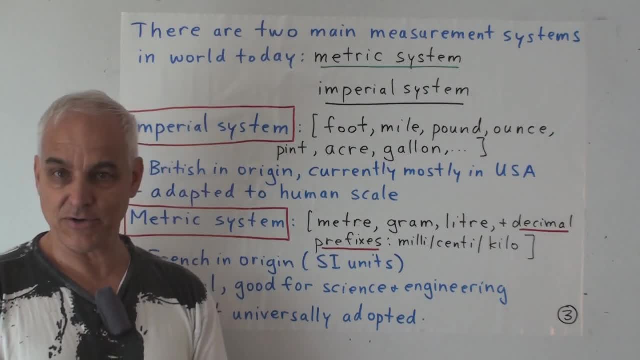 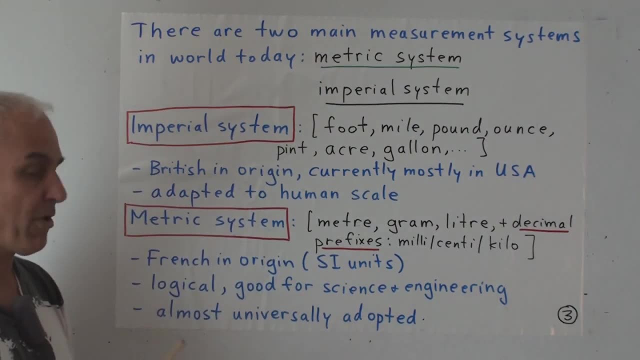 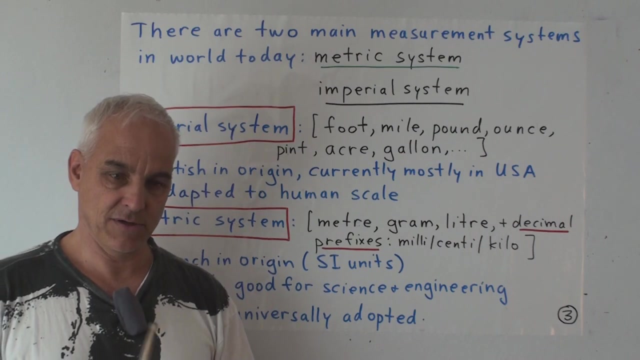 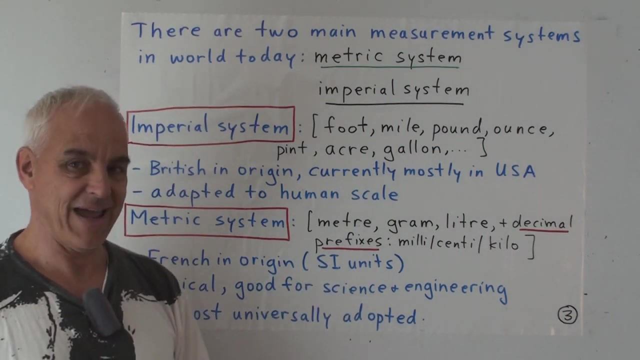 Revolution, when the French kicked out their aristocracy, chopped off the heads of the king and various others and instituted this more democratic logical system. It was actually one of Napoleon's first accomplishments was to institute this metrical system, And the system is often referred to in terms of SI units. So it's a logical system. It's very well. 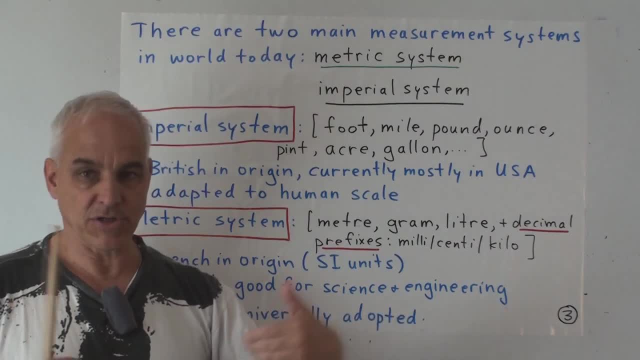 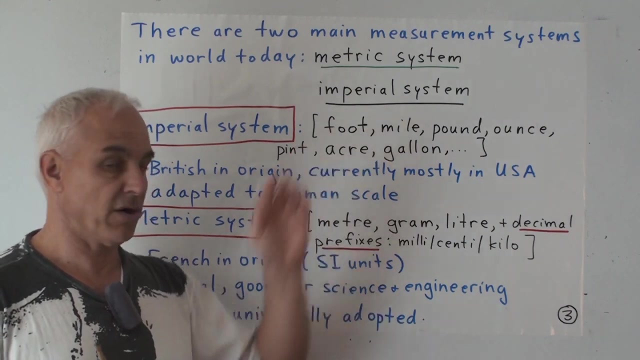 suited for science and engineering, And the fact that the powers of 10 play an important role means that it's well suited for the arithmetic of our number system. So, undoubtedly, doing calculations with the metrical system is easier than with the imperial system And, as I've said, it's almost universally adopted. 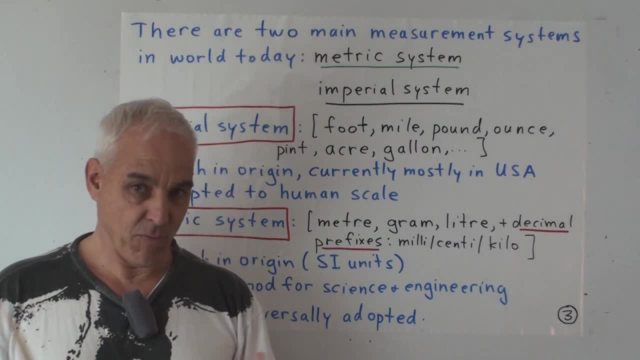 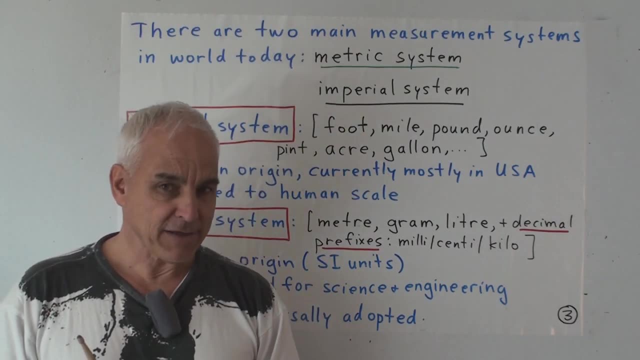 So you might think that from what I've said, I'm going to adopt the position that we're just going to work with the metrical system because it's far superior. In fact, I don't have such a strong position as that. I think that. 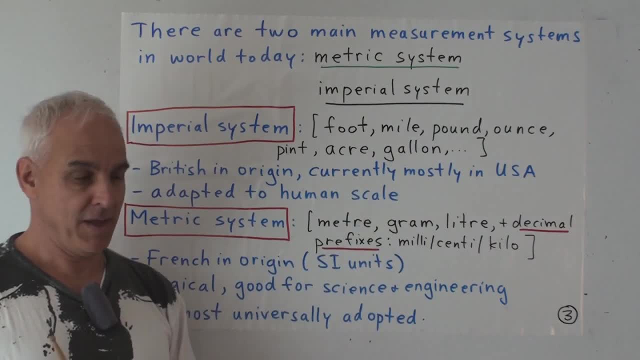 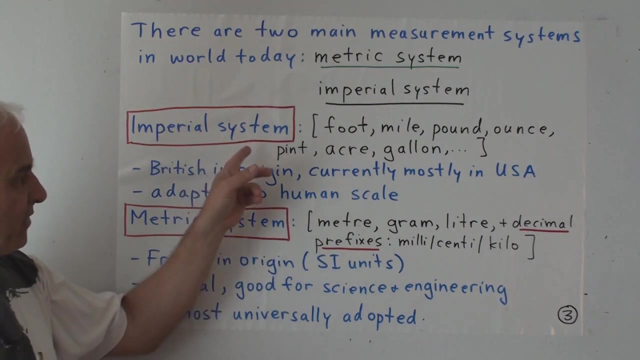 there are merits in both systems, in fact, And the- the metrical system- is not, in my view, perfect at all. In fact, it's a little bit unfortunate which units have been chosen. They didn't do such a good job, in my opinion. When you look more carefully, you see that a lot of the units in the 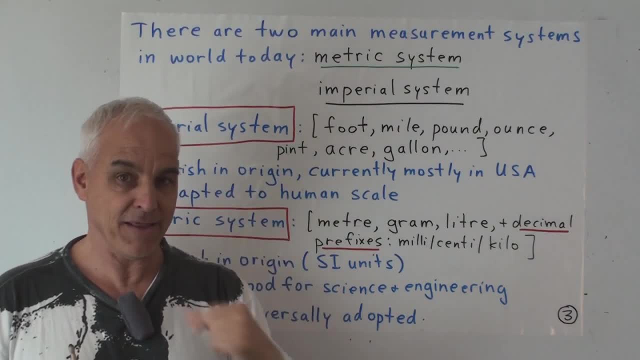 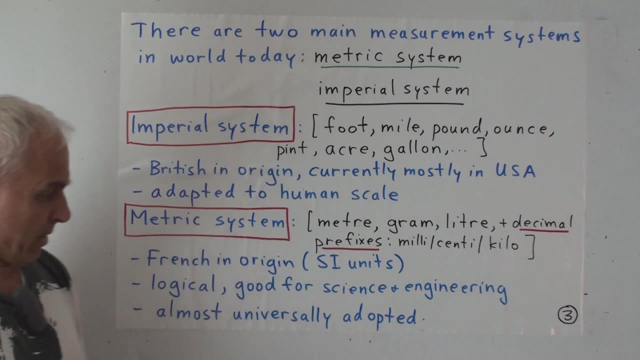 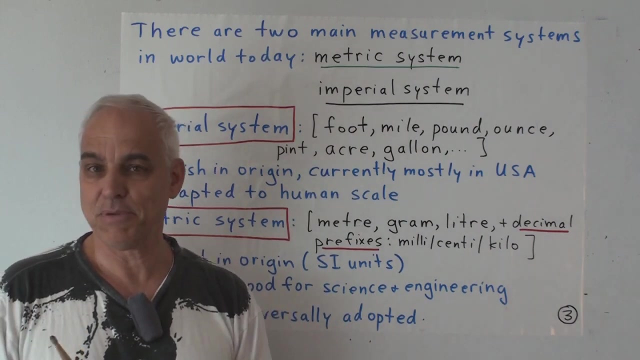 imperial system are actually more sensibly chosen than in the metrical system, And this is only my opinion, but we'll talk about that a little bit later. But because this is an international video series, I want to make it accessible to people all around the world. 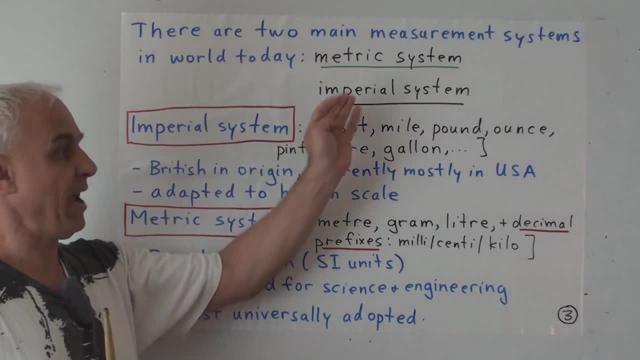 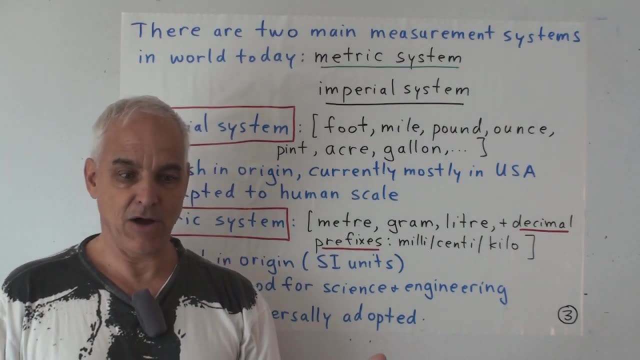 And so I'm going to be using both the metrical system and the imperial system for our examples. This is not bad and teaches young people how to, how to think about different systems, how to convert from one system to another. It's a very 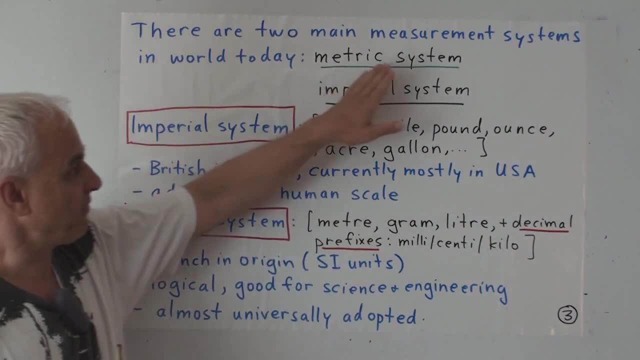 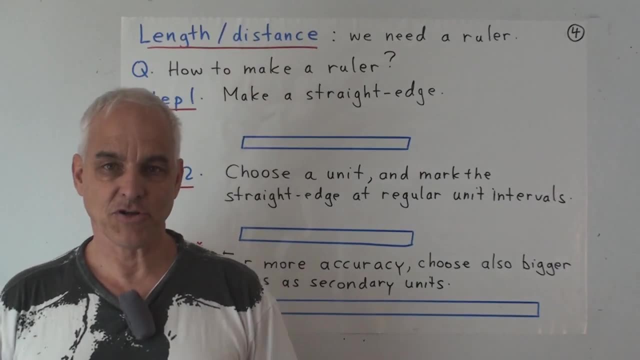 important skill. So we're going to be using some examples from the metric system and also some examples from the imperial system. Alright, so let's start with a discussion of length and distance. So the first thing that we need to do is we need to have a ruler. A ruler is something. 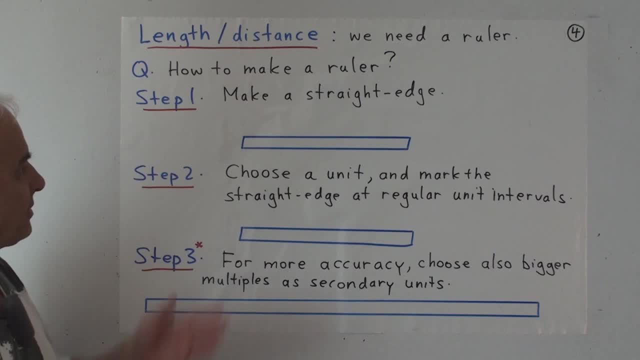 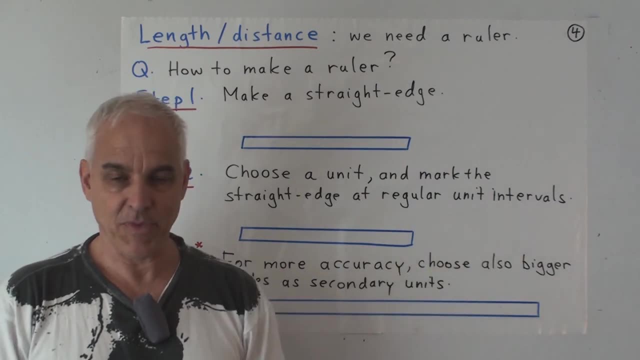 that measures length for us. And a good initial question is: how do we make a ruler? Of course these days you can go into a shop and buy them, but a thousand years ago you couldn't do that. If you wanted a ruler, you had to make one, And making a. 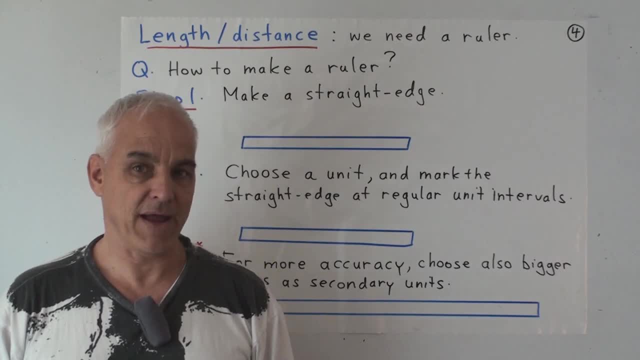 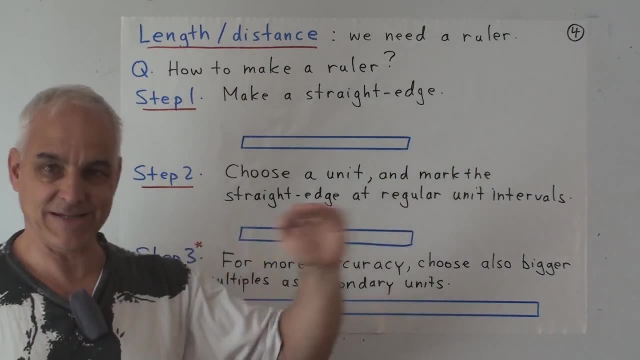 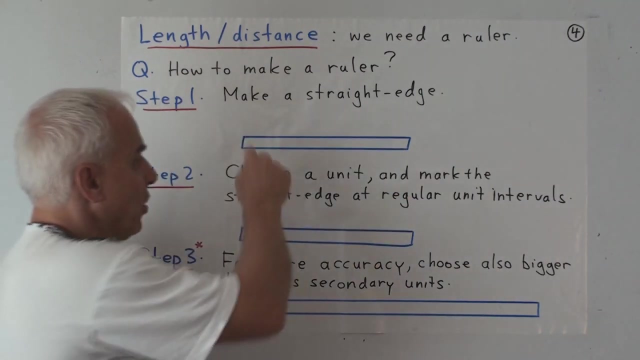 ruler is instructive and not at all that easy. The first step is that you need a straight edge. You need something that has a straight edge, a piece of wood, typically, that's been planed so that one at least edge is flat. Okay, how to do? that is a. 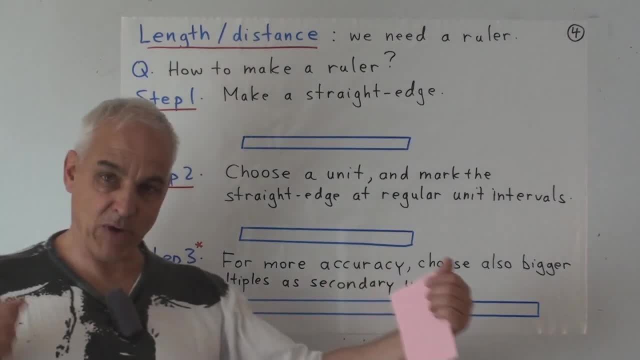 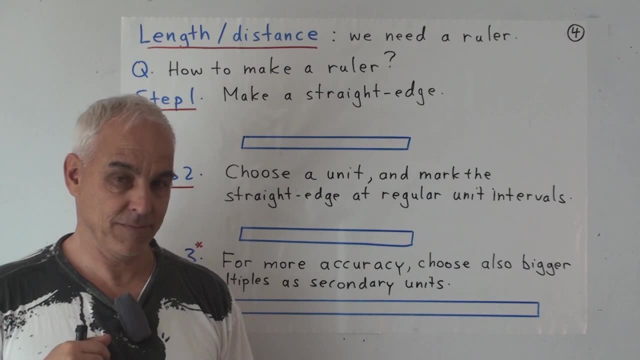 technical question. I remind you that if you want something that's straight, one way of getting something that's straight is to take a piece of string and tighten it. That way you get a straight line. So suppose we've gotten a straight edge and now we 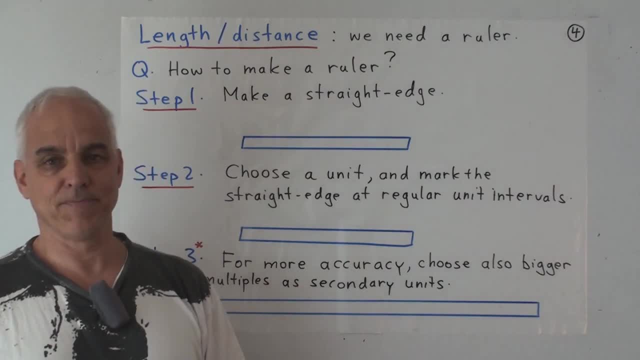 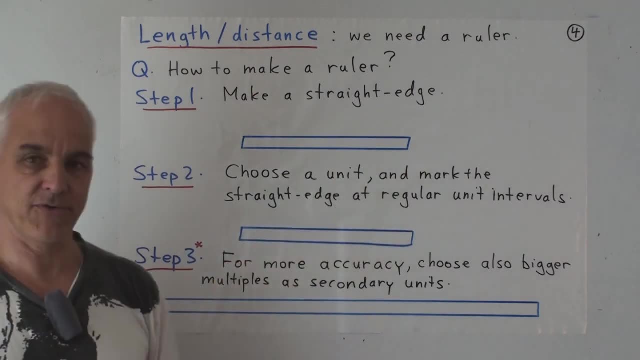 want to make markings on it which will serve us as a ruler. How are we going to do that? Well, we're going to choose a unit and we're going to mark the straight edge at regular unit intervals. So let's do that to this straight edge here, And I'm going to use this piece. 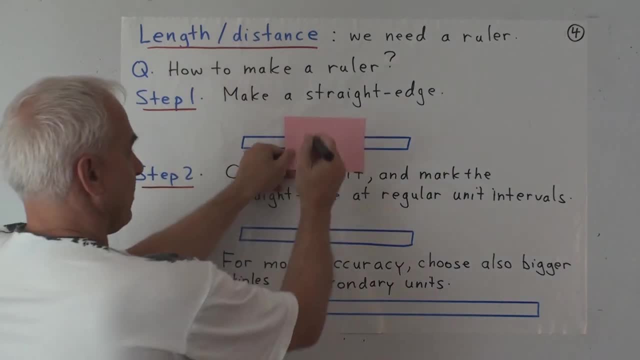 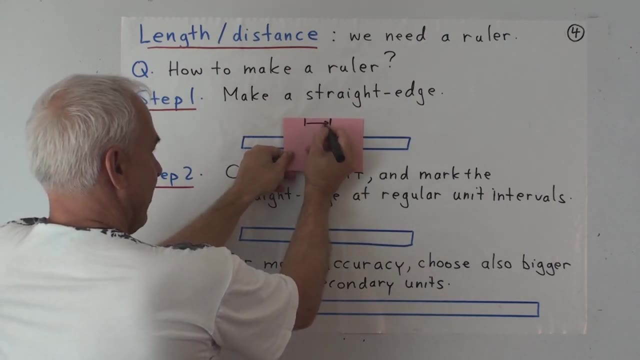 of paper here and I'm going to rather arbitrarily make a unit. So let's say that I'm going to call that separation one unit. I'm not going to give it a name because it's not going to be important for us, But I'm 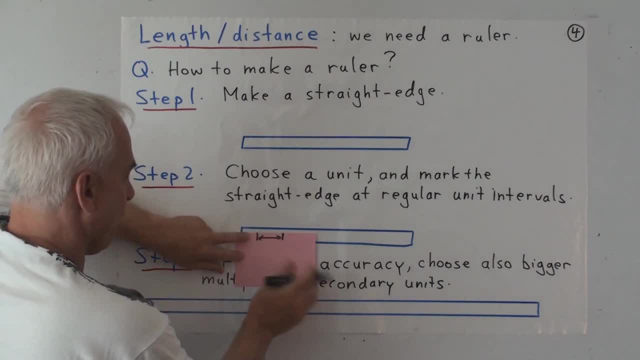 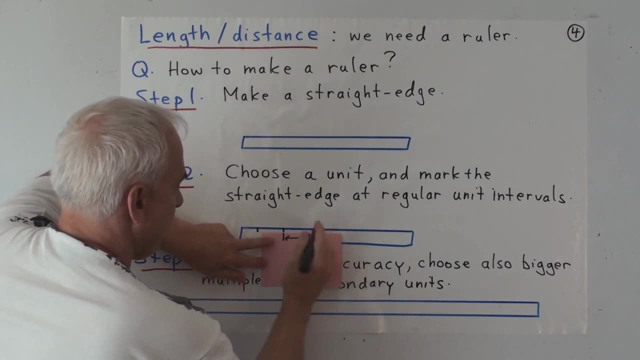 going to use this to mark our ruler. So what I'm going to do is I'm going to make a mark there and a mark there, say, And then I'm going to move this over until that's lined up again, so I can make another mark there. Now these are equally spaced. I'm going to move this. 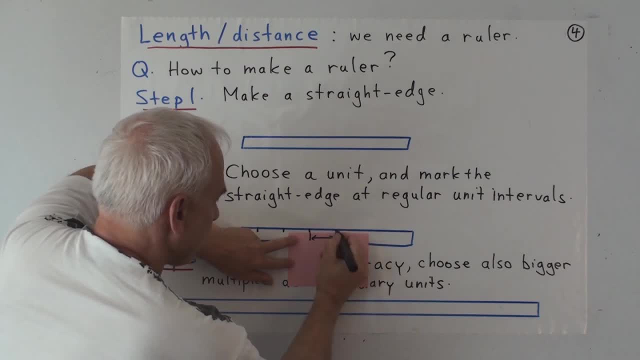 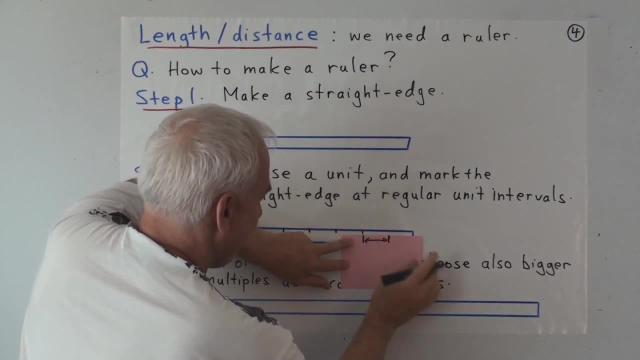 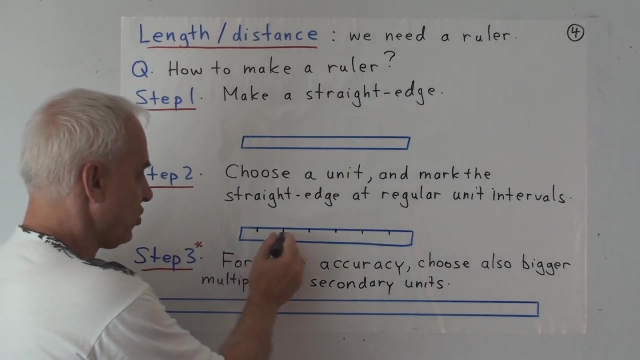 over again, Make another mark, And then another one, And then another one, And then another one, And I guess I've run out Alright. so there we have a primitive ruler that has one, two, three, four, five, six markings on it, And hopefully they're all equally spaced. 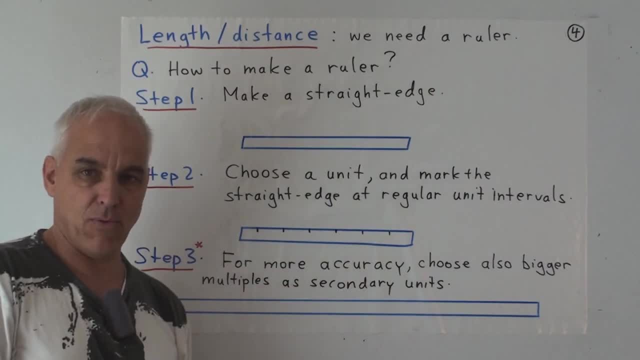 Or they're more or less equally spaced, depending on how accurate I was with my lines and how carefully I drew them and how carefully I lined them up. Alright, so of course that might not be a fine enough ruler. We might want to subdivide the. 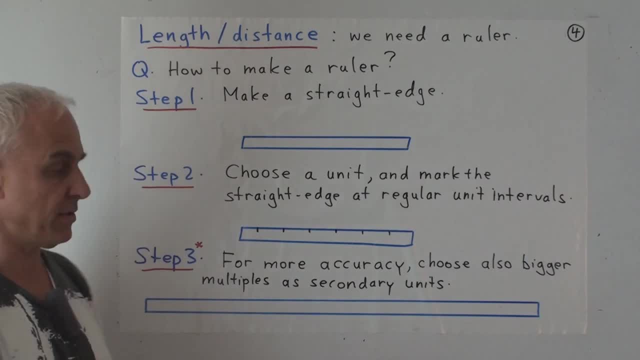 things. Or we may want to start with a smaller unit. So we could start with a smaller unit, Like suppose, for example, we wanted a unit that was that size, We could start with that and then repeat that. But that might not be as accurate as actually taking an existing. 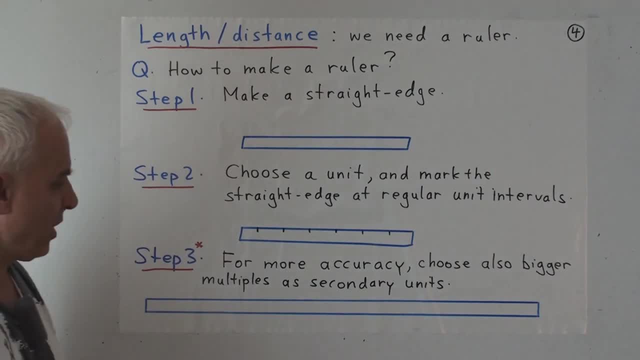 ruler like this and subdividing each one of its pieces. So, for example, if I take this thing here and I figure out where the halfway point is- I may have to make some construction to do that- Then I can use this to make a halfway point. 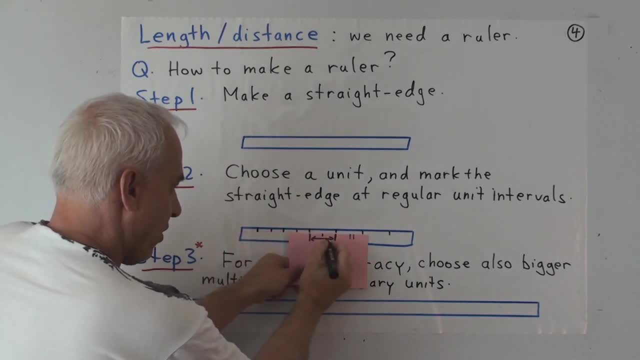 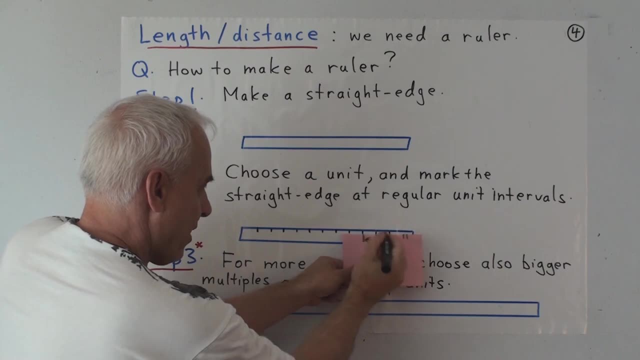 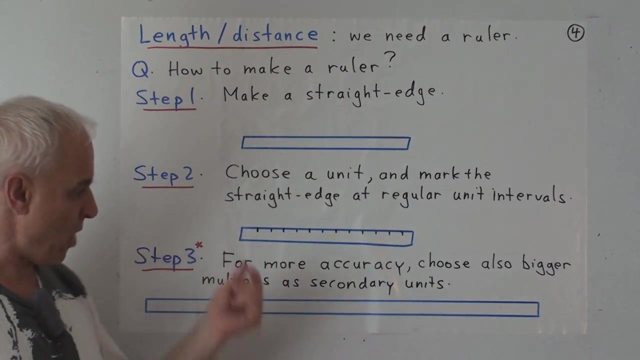 On all my little segments, So they're all sort of looking the same. Okay, now I've got a finer ruler than I had before, One with more subdivisions. I can be a little bit more accurate with this ruler, And the more subdivisions I have, well, the more accurate I get. 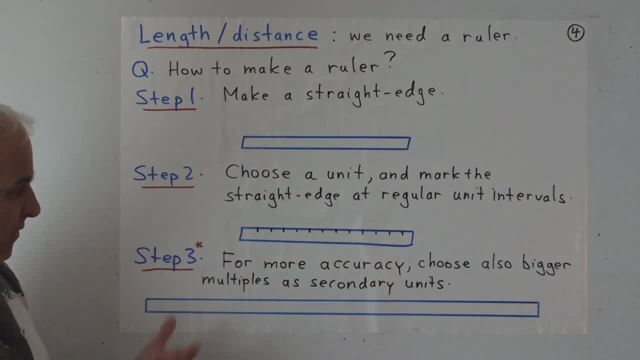 So that's good, And we've got a ruler now this size, But maybe we want a bigger ruler, Say one like this. Well then we could repeat the same process for that. But what we could also do is we could use our existing ruler. So suppose that this ruler here is really 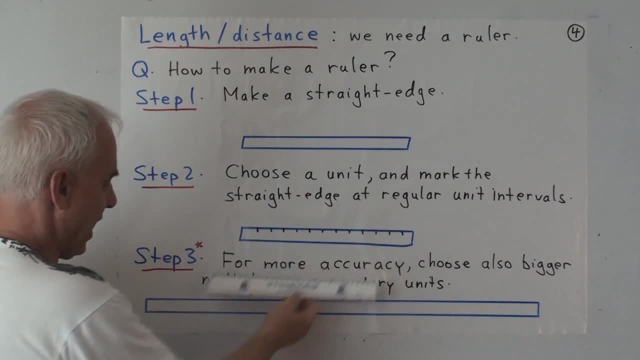 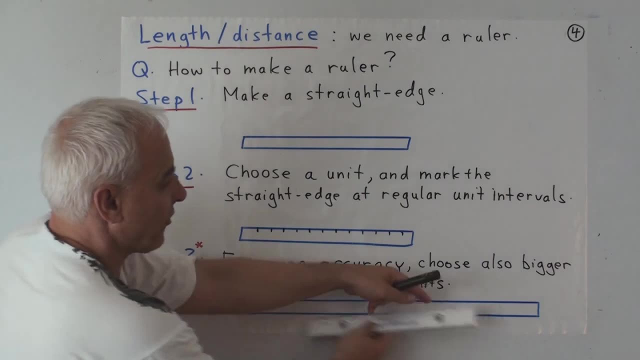 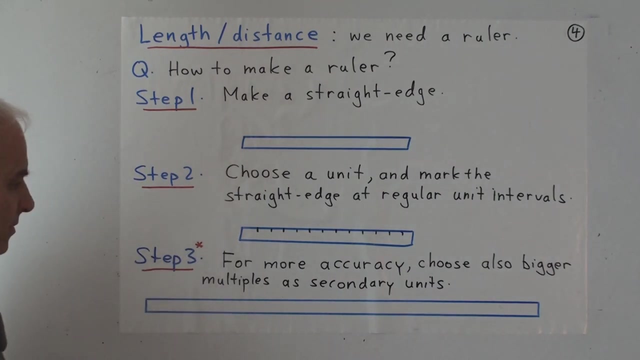 a copy of that one So I could use the existing ruler and then come down here And if you're essentially copy this one several times to make a more consistent, longer ruler, I'm just going to do that here. I'm going to use inches, which is in the imperial system. 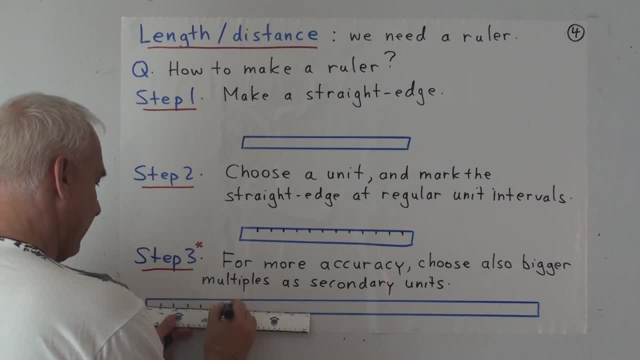 So there's 1,, 2,, 3,, 4,, 5,, 6,, 7,, 8,, 9,, 10,, 11, 12.. So I've used the ruler once, Then I come over here. Now I'm going to repeat. 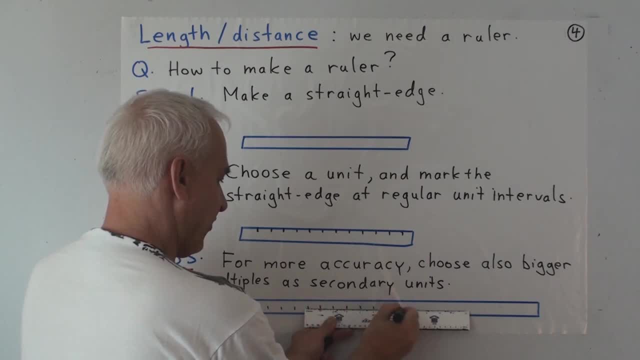 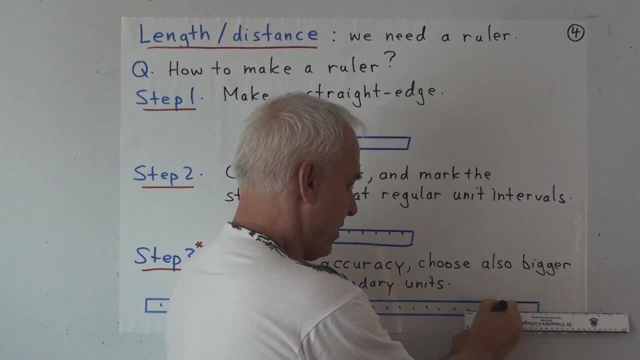 1,, 2,, 3,, 4,, 5,, 6,, 7,, 8,, 9,, 10,, 11,, 12.. And 1,, 2,, 3,, 4,, 5.. Okay, there is a ruler marked in imperial inches. So there is a ruler marked in imperial inches And with a ruler like this or a ruler like this, then we are in a position to go out and measure things. So let's have a look at this. 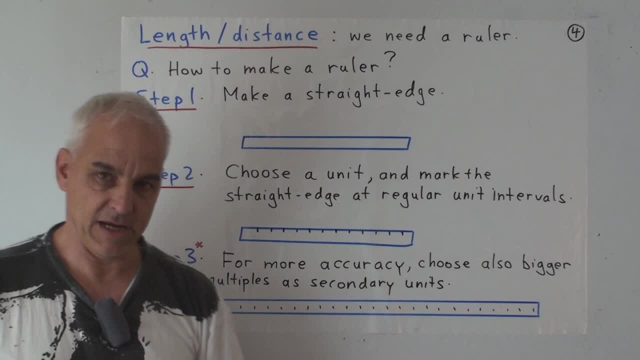 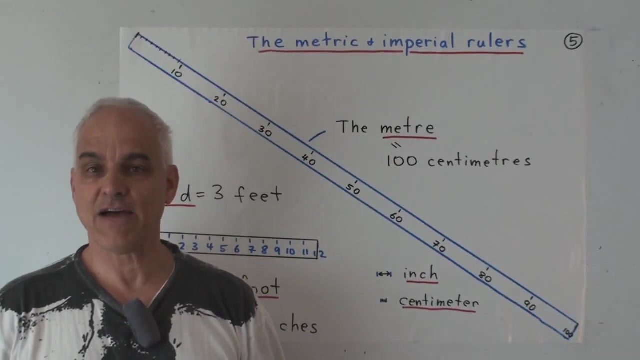 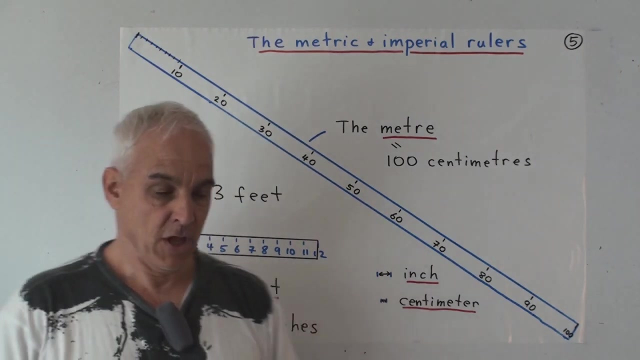 Okay, there is a ruler marked in imperial inches. So there is a ruler marked in imperial inches And with a ruler like this or a ruler like this, then we are in a position to go out and measure things. So let's have a look at 2 rulers from the two main systems: the imperial system and the metric system. So I've already shown you essentially a imperial system ruler. This is a foot rule. 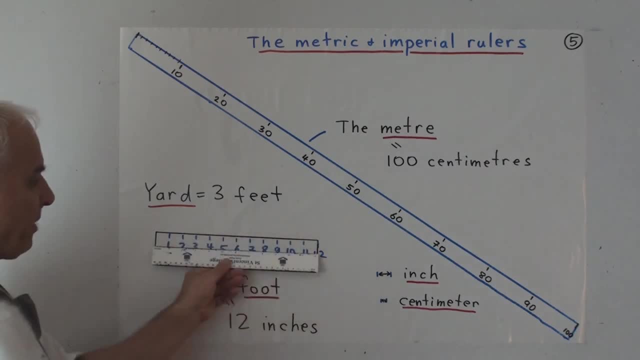 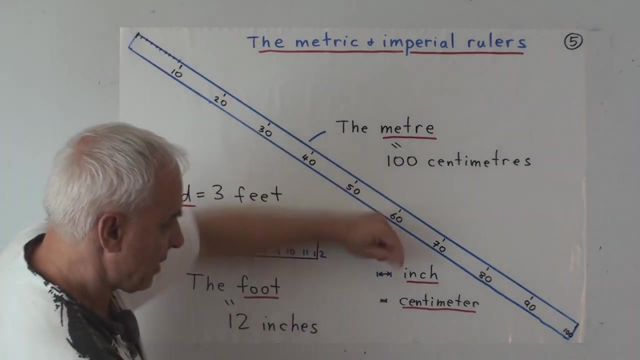 ruler and I've essentially copied it here. so that's imperial foot and it's composed of 12 subunits called inches. so there are 12 inches in the foot and here's roughly how an inch looks like. it's about the width of a thumb, one inch. 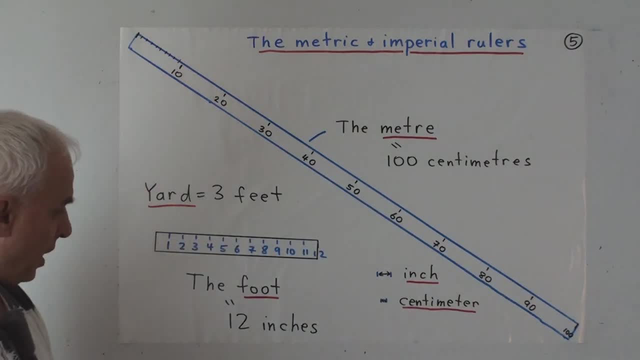 there 12 inches to make a foot. there's also a larger unit called the yard. the yard is exactly three feet. so if I took one here and I put another one here and then another one there, then I would get a yard. maybe if I start here, maybe I'll. 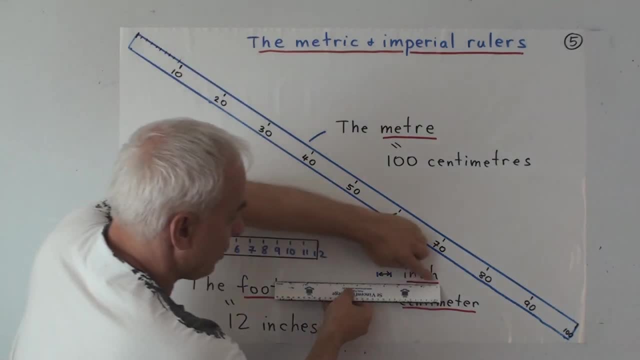 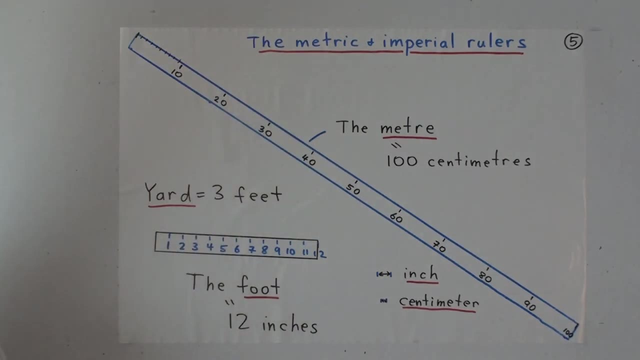 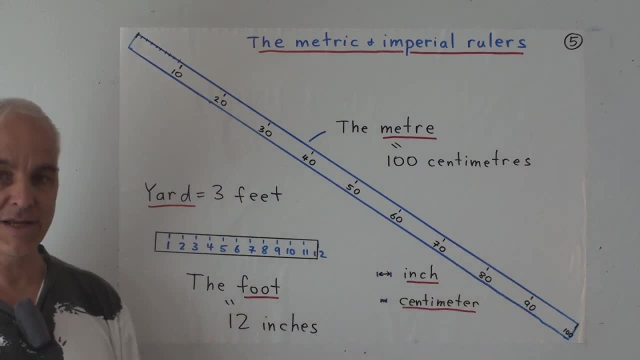 this the width of this sheet here. those, this the width of this sheet here. those are the three fundamental. short are the three fundamental. short are the three fundamental short measurements in the imperial system. the measurements in the imperial system. the measurements in the imperial system: the inch, the foot and the yard in the. 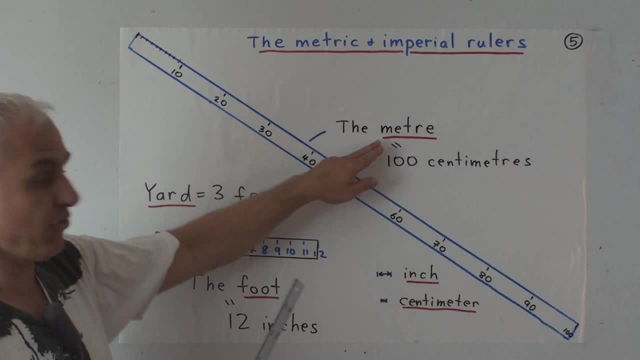 inch the foot and the yard in the inch the foot and the yard in the metrical system. the main unit is the metrical system. the main unit is the metrical system. the main unit is the meter, which is that long, and here is a meter which is that long and here is a. 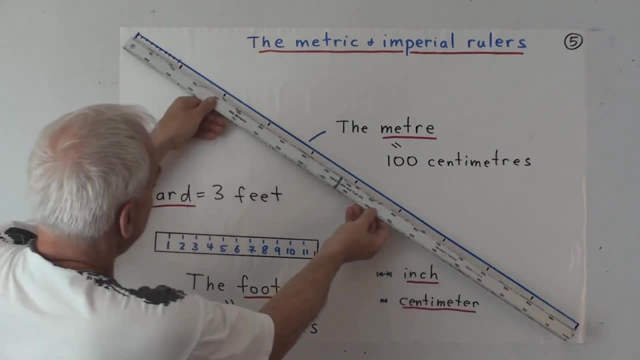 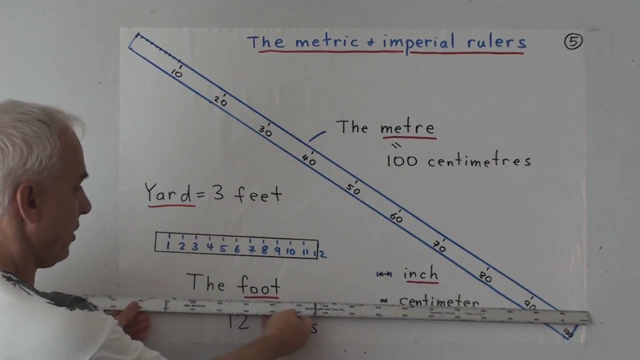 meter, which is that long. and here is a meter ruler there, it is right there. meter ruler there, it is right there. meter ruler there, it is right there. all right, that's one meter long. it's a. all right, that's one meter long. it's a. all right, that's one meter long. it's a little bit longer than a yard you can. 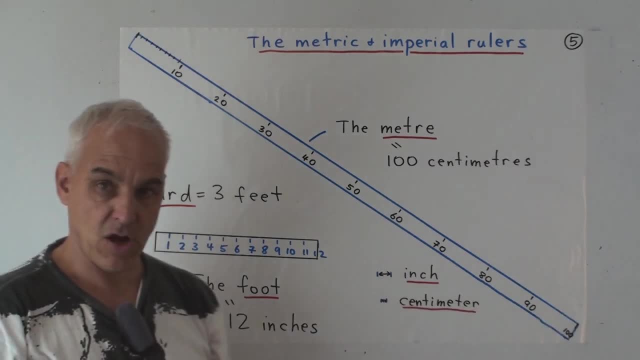 little bit longer than a yard you can, little bit longer than a yard you can see. it's about that much longer about see. it's about that much longer about see. it's about that much longer, about three inches longer than a yard, but three inches longer than a yard. but 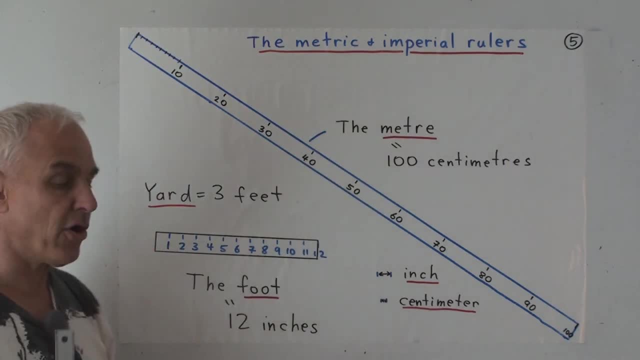 three inches longer than a yard, but they're pretty close and both the yard they're pretty close and both the yard they're pretty close and both the yard and the meter are suited to outdoor and the meter are suited to outdoor and the meter are suited to outdoor measurement because they represent a 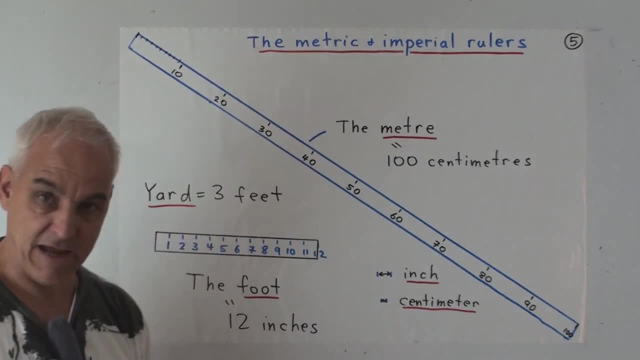 measurement, because they represent a measurement, because they represent a man's pace. so if you take a reasonable man's pace, so if you take a reasonable man's pace, so if you take a reasonable size step, then you're getting pretty. size step, then you're getting pretty. 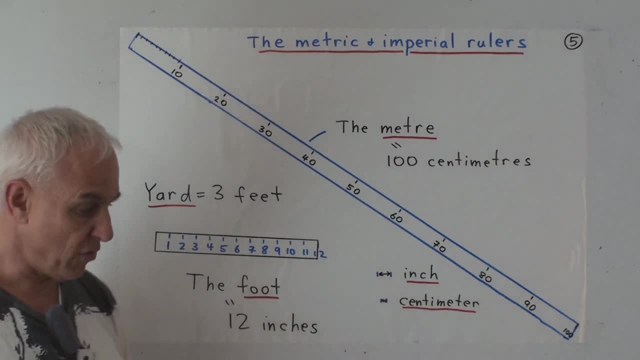 size step, then you're getting pretty close to a yard or a meter. and so if you close to a yard or a meter, and so if you close to a yard or a meter, and so if you want to measure out a field, or want to measure out a field or 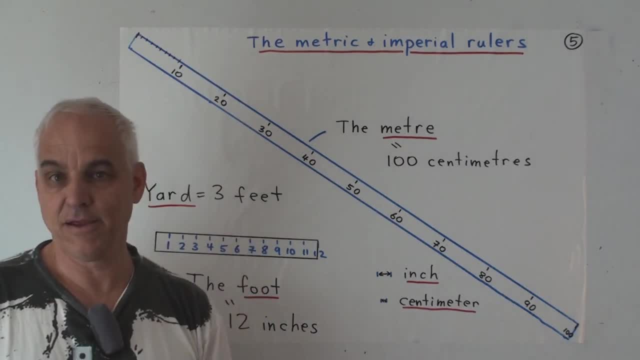 want to measure out a field or something. well, you just pace it out and something. well, you just pace it out and something. well, you just pace it out and you're getting the the length of that, you're getting the the length of that. you're getting the the length of that field in meters. so it's very natural. 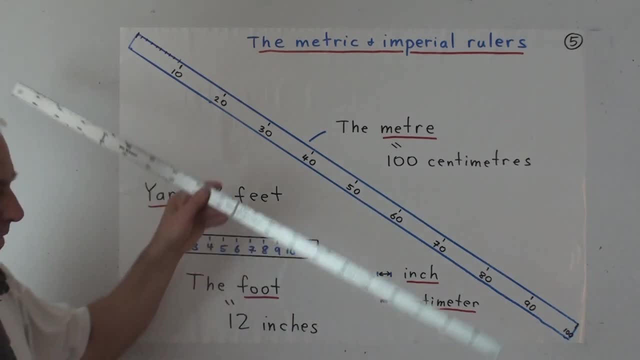 field in meters, so it's very natural. field in meters, so it's very natural. unit for outdoor activity, of course, for unit for outdoor activity, of course, for unit for outdoor activity, of course for indoor activity, this is rather long unit. indoor activity, this is rather long unit. 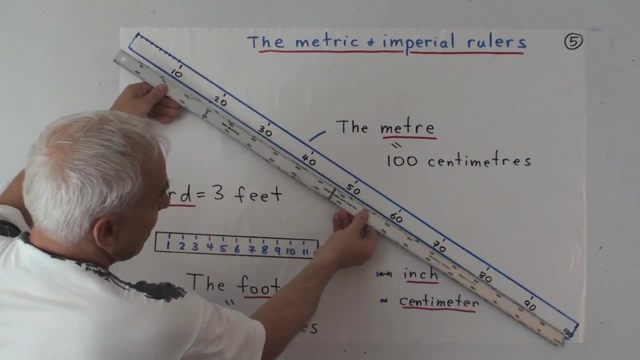 indoor activity. this is rather long unit, but we can subdivide it. and in the but we can subdivide it. and in the but we can subdivide it. and in the metric system we always subdivide by metric system. we always subdivide by metric system. we always subdivide by dividing by 10, not by 12 or anything. 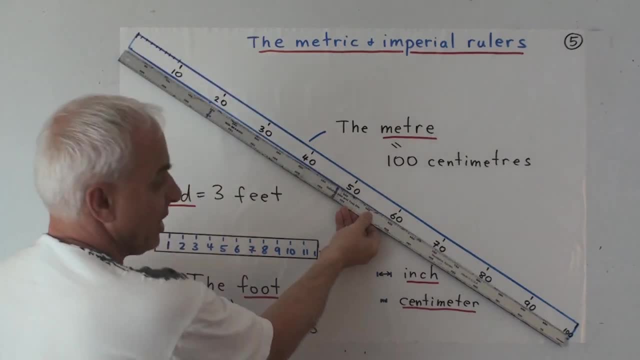 dividing by 10, not by 12 or anything. dividing by 10, not by 12 or anything else, always by 10. so here we've else, always by 10. so here we've else, always by 10. so here we've subdivided the meter into 10 units, but I 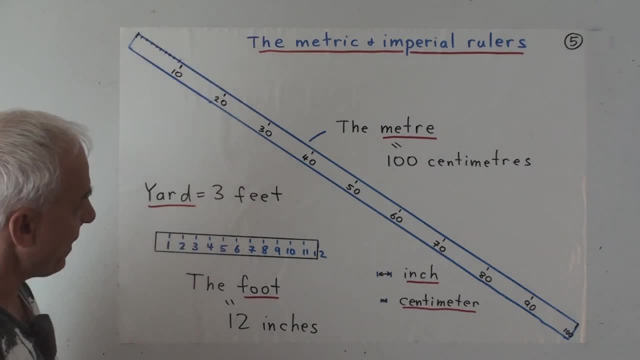 subdivided the meter into 10 units. but I subdivided the meter into 10 units but I haven't marked them. 1, 2, 3, I've marked. haven't marked them. 1, 2, 3, I've marked. haven't marked them 1, 2, 3, I've marked them 10, 20 and 30. another reason is: 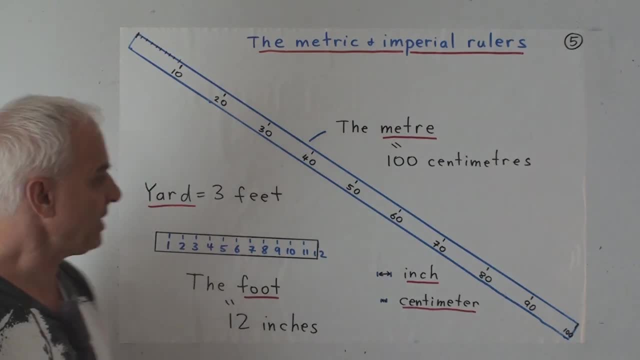 them 10, 20 and 30. another reason is them 10, 20 and 30. another reason is because, for some historical reason, this, because for some historical reason, this, because for some historical reason, this unit which is a decimeter is almost. unit which is a decimeter is almost. 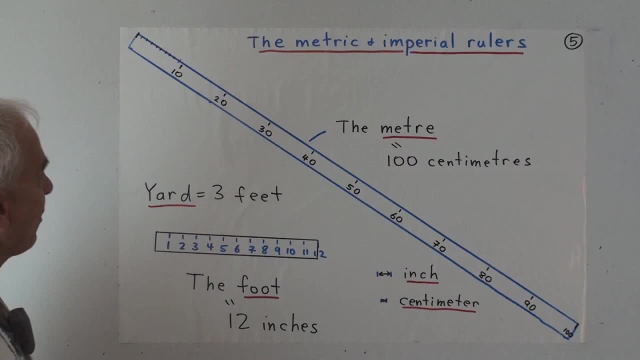 unit which is a decimeter, is almost never explicitly used, rather, we think never explicitly used, rather, we think never explicitly used. rather, we think about 1 tenth of it, which is called a, about 1 tenth of it which is called a, about 1 tenth of it which is called a centimeter. so a centimeter is about this. 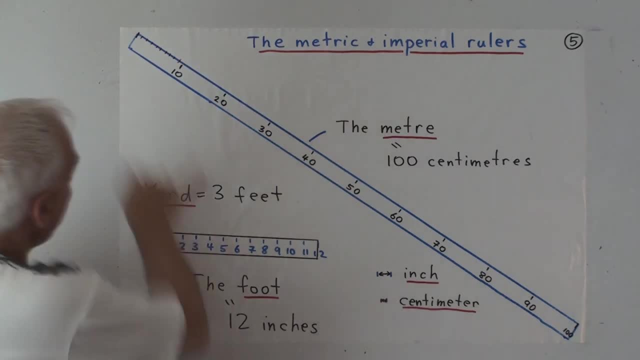 centimeter. so a centimeter is about this centimeter. so a centimeter is about this big. it's about the size of a little big. it's about the size of a little big. it's about the size of a little finger, and there are 10 of them that fit. 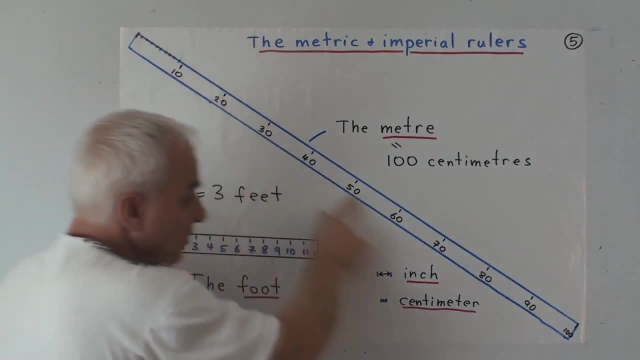 finger and there are 10 of them that fit finger and there are 10 of them that fit inside a decimeter and there are 100 of inside a decimeter and there are 100 of inside a decimeter and there are 100 of them that fit inside a meter. so most 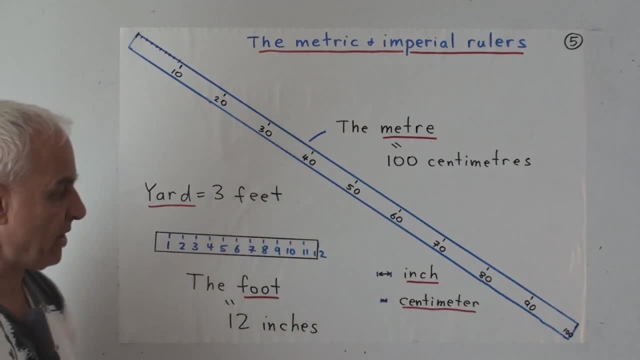 them that fit inside a meter. so most them that fit inside a meter. so most measurements say in a house, in the measurements say in a house. in the measurements say in a house, in the metrical system will use centimeters. metrical system will use centimeters. 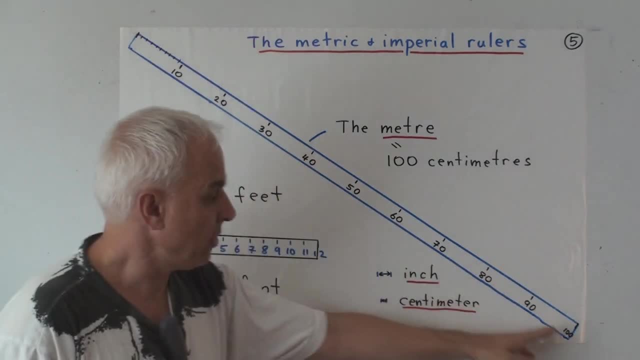 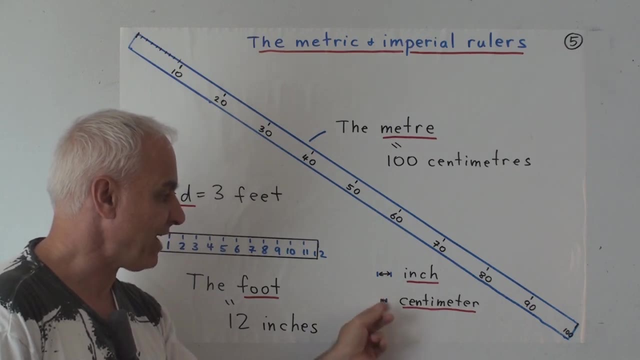 metrical system will use centimeters, which are this big, or meters, which are, which are this big, or meters, which are, which are this big, or meters, which are this big. there's also a smaller unit this big. there's also a smaller unit this big. there's also a smaller unit called a millimeter. if we divide a, 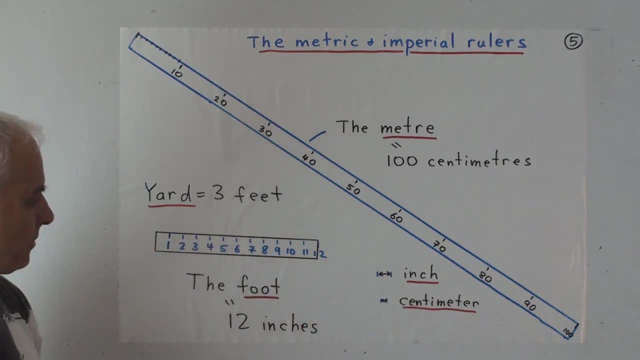 called a millimeter. if we divide a called a millimeter. if we divide a centimeter by 10, we get a millimeter. centimeter by 10, we get a millimeter. centimeter by 10, we get a millimeter. alright, so we have these two systems. 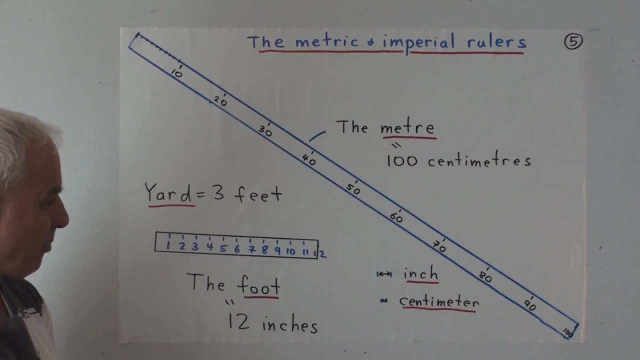 alright, so we have these two systems. alright. so we have these two systems here and now. perhaps it's it's it's here and now. perhaps it's it's here and now, perhaps it's it's. it's appropriate for me to say that it's not. 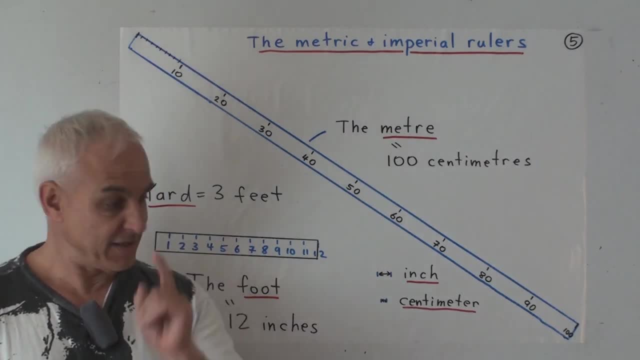 appropriate for me to say that. it's not appropriate for me to say that it's not at all clear that this metrical choice at all clear that this metrical choice at all clear that this metrical choice is superior, it's superior in terms of is superior, it's superior in terms of. 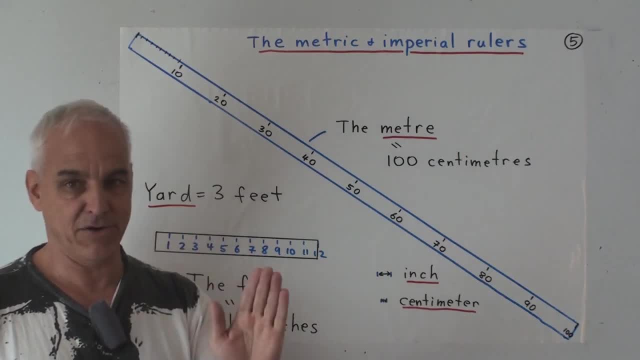 is superior. it's superior in terms of the powers of 10 involved. that clearly the powers of 10 involved, that clearly the powers of 10 involved. that clearly is more logical than dividing something is more logical than dividing something is more logical than dividing something by 12 or using a multiple of 3. so 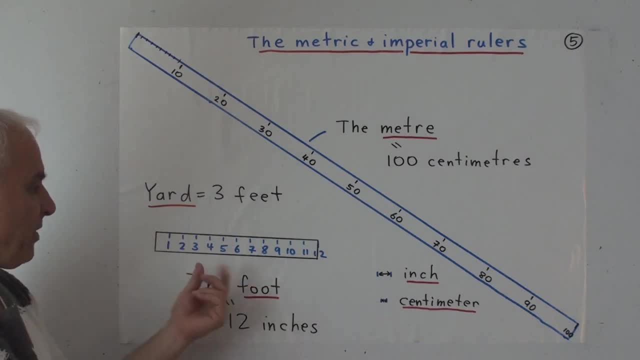 by 12 or using a multiple of 3. so by 12 or using a multiple of 3. so there's an arbitrariness here in the in. there's an arbitrariness here in the in. there's an arbitrariness here in the in the Imperial system that we divided the. 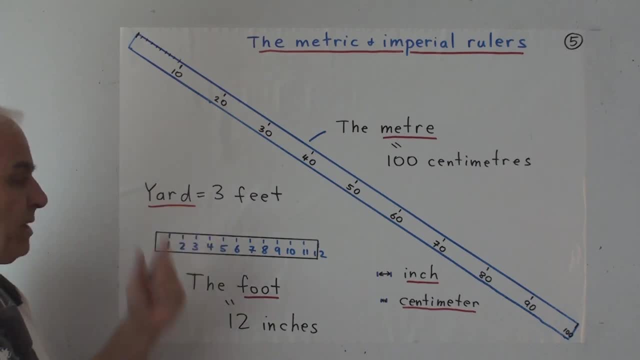 the Imperial system, that we divided the the Imperial system, that we divided the foot into 12 units, and that we've foot into 12 units and that we've foot into 12 units and that we've chosen 3 feet to be equal to 1 yard. but 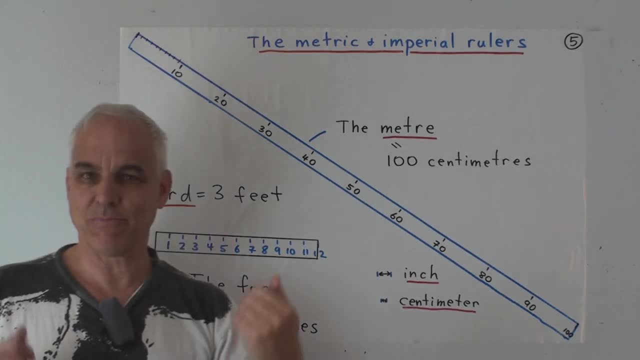 chosen 3 feet to be equal to 1 yard, but chosen 3 feet to be equal to 1 yard. but the inch, the foot and the yard are much the inch. the foot and the yard are much the inch. the foot and the yard are much better suited for length measurements for 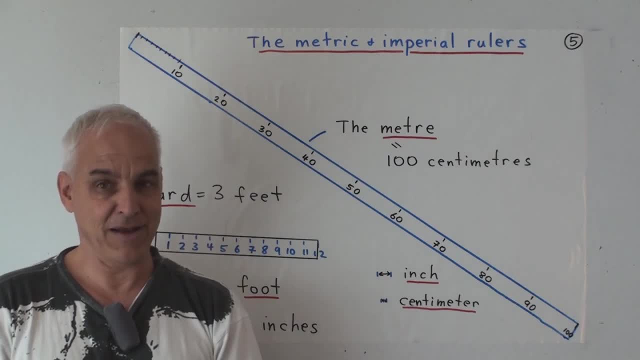 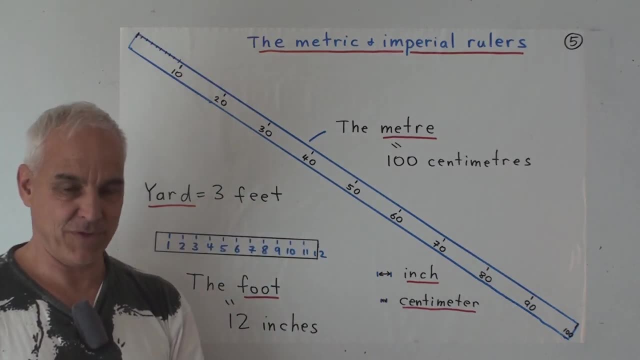 better suited for length measurements for better suited for length measurements for human beings. this is the reality for human beings. this is the reality for human beings. this is the reality for many applications. these measurements are many applications. these measurements are many applications. these measurements are are easier and more natural. they're. 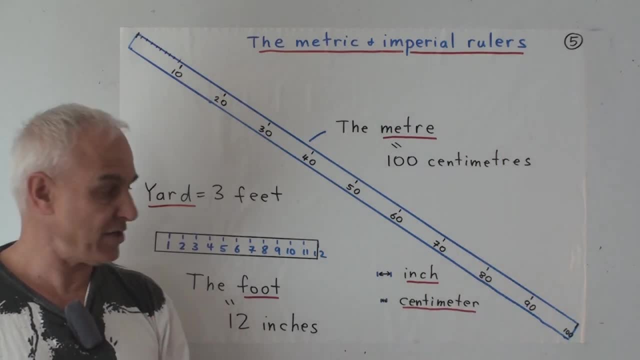 are easier and more natural. they're are easier and more natural. they're just the sizes of them are are easier. us just the sizes of them are are easier. us just the sizes of them are are easier. us much more manageable than a centimeter. much more manageable than a centimeter. 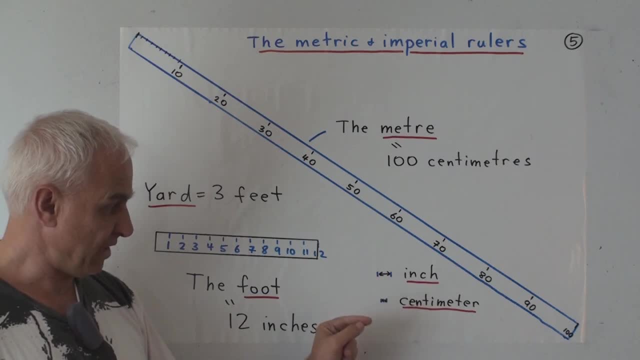 much more manageable than a centimeter. not much of a difference. an inch is two. not much of a difference. an inch is two. not much of a difference. an inch is two and a half centimeters, but it's a and a half centimeters, but it's a. 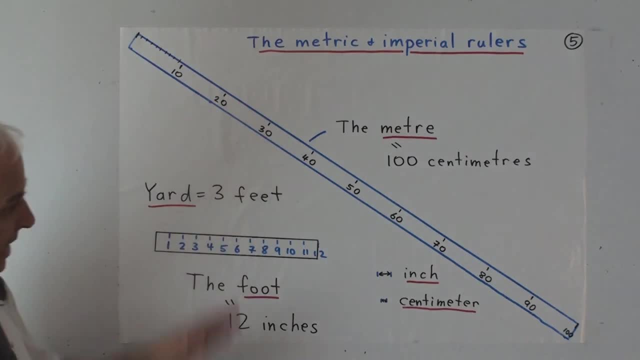 and a half centimeters, but it's a noticeable difference. when you're noticeable difference, when you're noticeable difference when you're measuring things, and again here you can measuring things. and again here you can measuring things. and again here you can see the meter. well, it's, it's, it's fine. 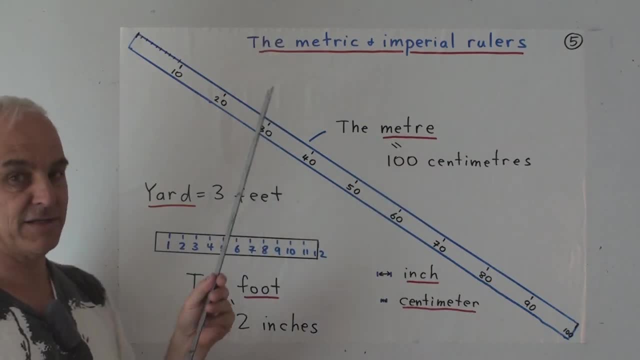 see the meter: well it's, it's, it's fine. see the meter: well it's, it's, it's fine. for outdoor activity, for indoor things. a for outdoor activity for indoor things. a for outdoor activity for indoor things. a meter is is too long, a foot is a much. 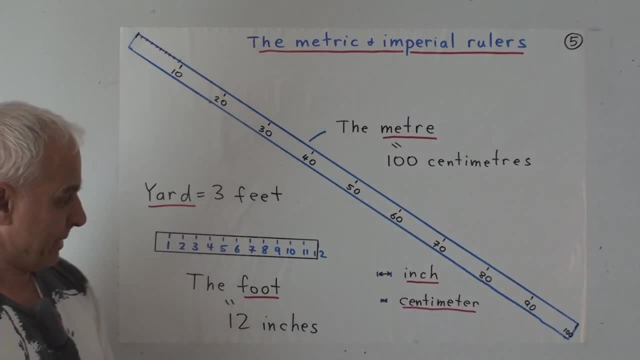 meter is is too long. a foot is a much meter is is too long. a foot is a much more manageable unit. so you know if I more manageable unit. so you know if I more manageable unit. so you know if I had a minute magic wand and I could wave. 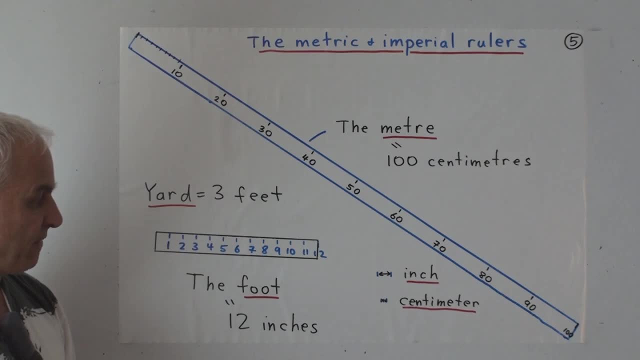 had a minute magic wand and I could wave. had a minute magic wand and I could wave it. I would change the decimal system so it. I would change the decimal system so it. I would change the decimal system so that the fundamental meter was not this, that the fundamental meter was not this. 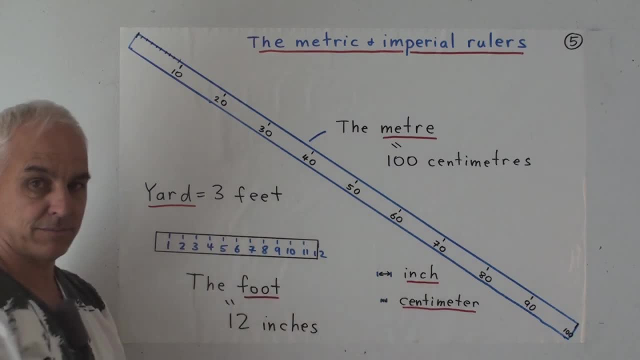 that the fundamental meter was not this long, but it was rather more like this long, but it was rather more like this long, but it was rather more like this long and I would say that a tenth of a long and I would say that a tenth of a. 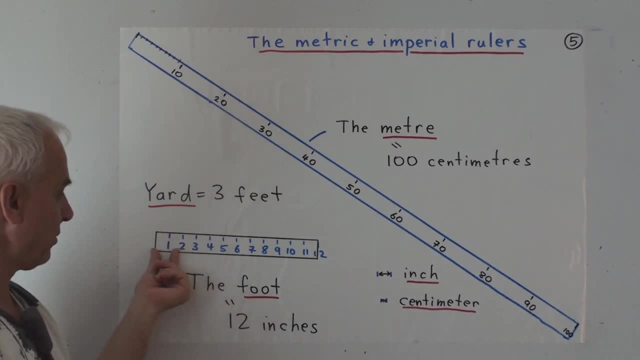 long and I would say that a tenth of a meter this kind of meter would be. would meter this kind of meter would be. would meter this kind of meter would be. would be given a name like an inch or a. be given a name like an inch or a. 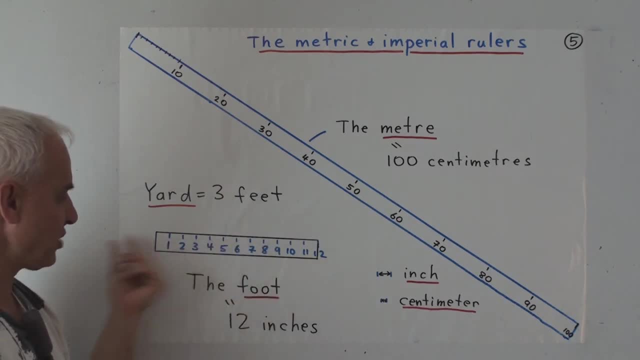 be given a name like an inch or a decimeter, but a tenth of this unit is decimeter. but a tenth of this unit is decimeter. but a tenth of this unit is quite natural. so an inch and a foot are quite natural. so an inch and a foot are. 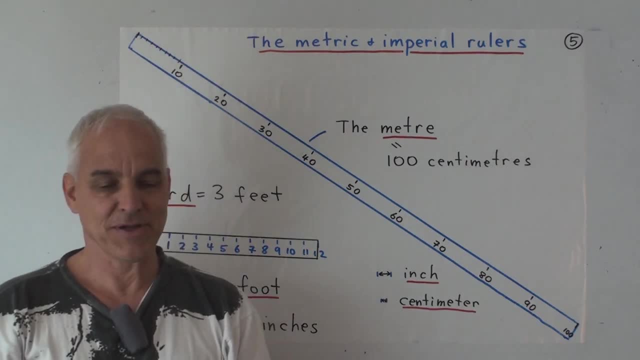 quite natural. so an inch and a foot are, in fact, quite natural. so that's not so, in fact, quite natural. so that's not so, in fact, quite natural. so that's not so. the, the case between Imperial and the the case between Imperial and the the case between Imperial and Metrical is not as cut and dried as the. 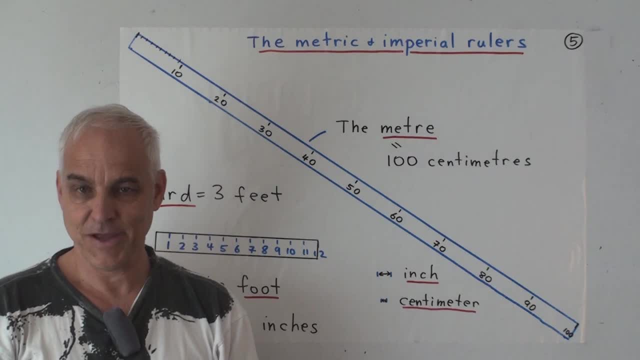 Metrical is not as cut and dried as the Metrical is not as cut and dried as the metrical proponents make it out to be so. metrical proponents make it out to be so. metrical proponents make it out to be so. we're going to measure in both systems. 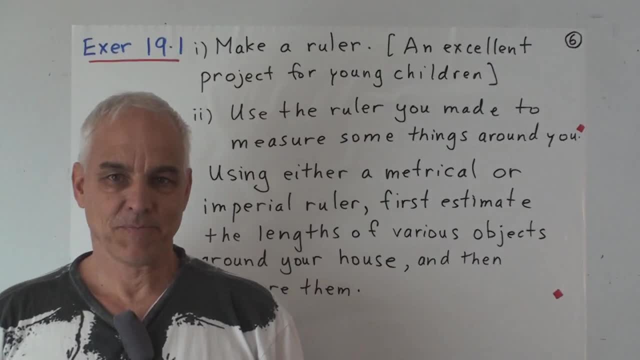 we're going to measure in both systems. we're going to measure in both systems in this in this course. so here are some in this in this course. so here are some in this in this course. so here are some exercises that you can do or you can do. 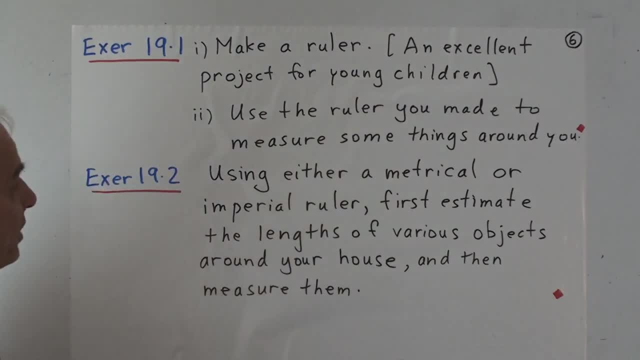 exercises that you can do or you can do, exercises that you can do or you can do with some young friends that you may with some young friends, that you may with some young friends that you may have, and the first one is to actually have, and the first one is to actually 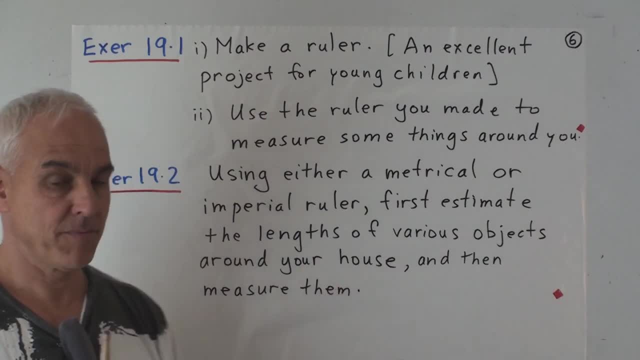 have, and the first one is to actually make a ruler actually physically make a make a ruler actually physically make a make a ruler actually physically make a ruler, and this is an excellent project ruler and this is an excellent project ruler and this is an excellent project for young children. get their hands doing. 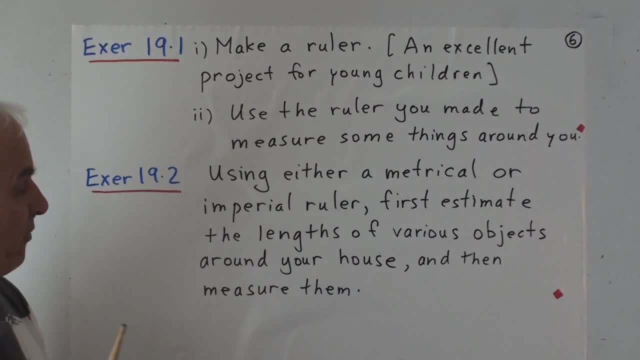 for young children, get their hands doing for young children, get their hands doing some handiwork making some markings and some handiwork making some markings and some handiwork making some markings. and then they have a ruler, the rulers don't. then they have a ruler, the rulers don't. 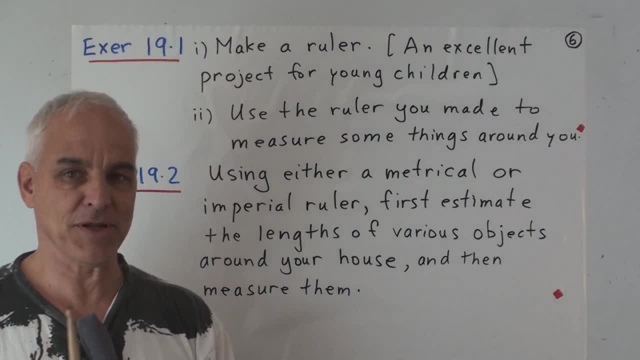 then they have a ruler. the rulers don't all have to be in the same units. let the all have to be in the same units. let the all have to be in the same units. let the children choose the units that they want. children choose the units that they want. 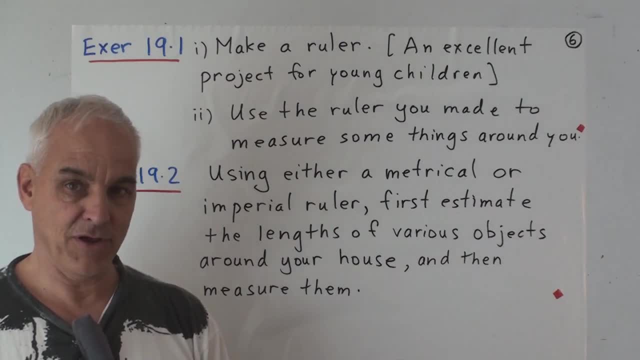 children choose the units that they want and they have their own personal units and they have their own personal units and they have their own personal units and they go around measuring things with and they go around measuring things with and they go around measuring things with their own personal units, and that's what. 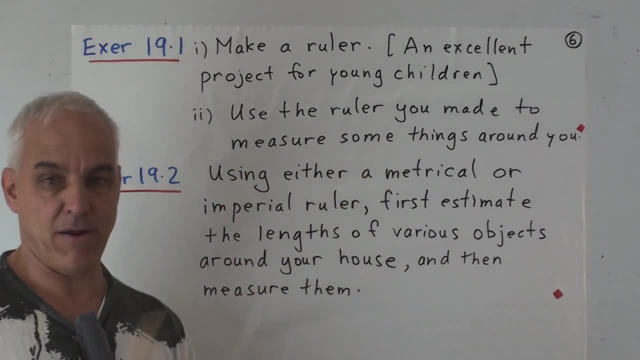 their own personal units, and that's what their own personal units and that's what they should do. they should use the ruler. they should use the ruler to measure some of the things around them, the to measure some of the things around them, the to measure some of the things around them. the second exercise is to use either a: 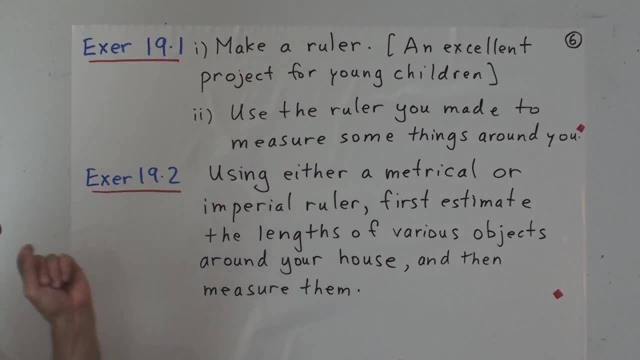 second exercise is to use either. a second exercise is to use either a metrical or imperial ruler. to first metrical or imperial ruler. to first metrical or imperial ruler. to first estimate the lengths of various objects. estimate the lengths of various objects. estimate the lengths of various objects around your house, both inside and 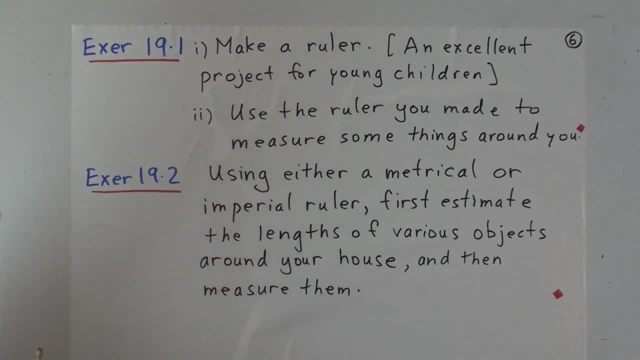 around your house, both inside and around your house, both inside and outside your house, or where you live and outside your house, or where you live and outside your house or where you live, and then try to make some measurements. see, then try to make some measurements. see, then try to make some measurements, see if you can figure out and compare your. 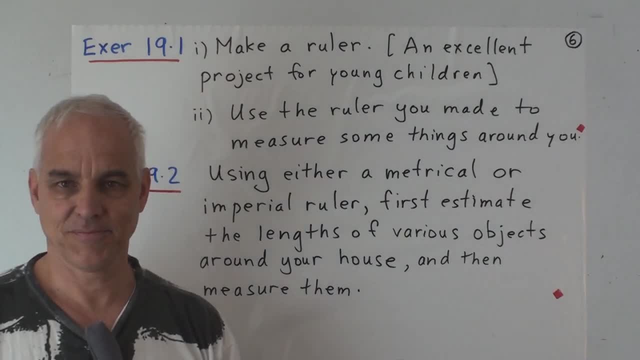 if you can figure out and compare your, if you can figure out and compare your guesses with the actual measurements. so, guesses with the actual measurements. so this kind of exercise where young, this kind of exercise where young, this kind of exercise where young people go out and actually make. 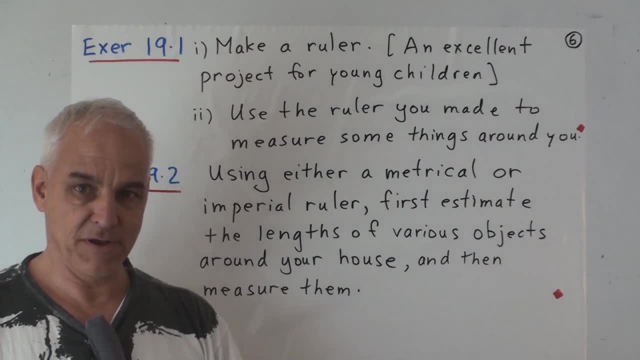 people go out and actually make people go out and actually make measurements is very important and measurements is very important and measurements is very important and important part of becoming scientific, important, part of becoming scientific, important part of becoming scientific. thinking well, there's there's guesses thinking, well, there's there's guesses. 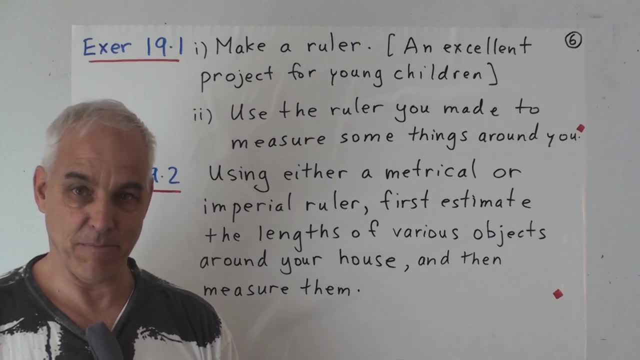 thinking: well, there's, there's guesses, and then there's measurements and they're, and then there's measurements and they're, and then there's measurements, and they're not always the same thing, the not always the same thing, the not always the same thing. the measurements are usually more. 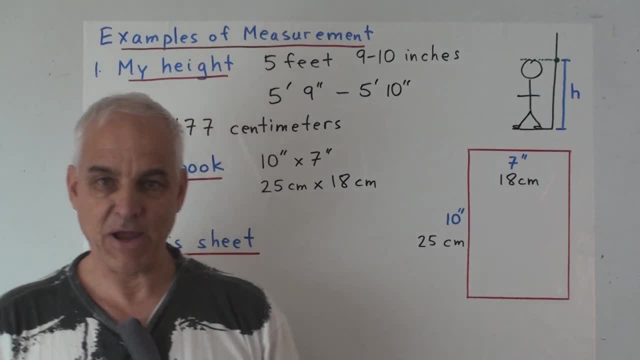 measurements are usually more. measurements are usually more trustworthy, all right. so let's do a trustworthy, all right, so let's do a trustworthy, all right. so let's do a little bit of measuring just ourselves, little bit of measuring just ourselves, little bit of measuring just ourselves. so here are some examples of measurement. 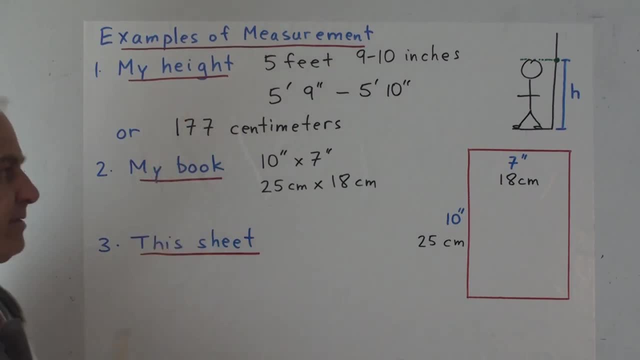 so here are some examples of measurement. so here are some examples of measurement. one natural thing to measure is my. one natural thing to measure is my. one natural thing to measure is my height. so to do that, I stand on the height. so to do that, I stand on the. 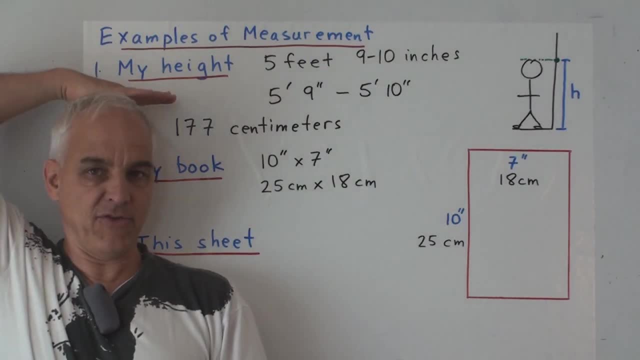 height. so to do that, I stand on the floor and I put my back against the wall floor, and I put my back against the wall floor and I put my back against the wall and I get a book or something like this. and I get a book or something like this. 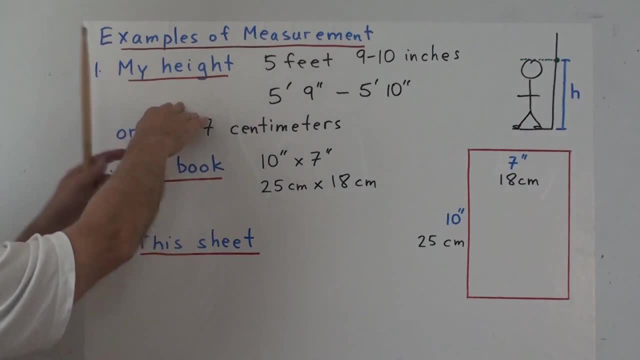 and I get a book or something like this, and I make a mark, make a mark there, and and I make a mark, make a mark there, and and I make a mark, make a mark there, and then I get my ruler and I measure how. then I get my ruler and I measure how. 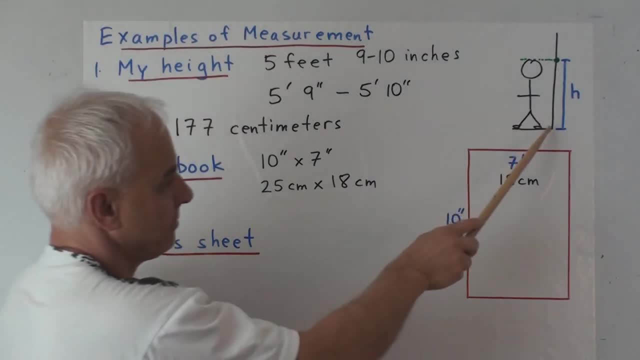 then I get my ruler and I measure how far it is from the ground to the mark. far it is from the ground to the mark. far it is from the ground to the mark that I made. that's the height H and my. that I made. that's the height H and my. 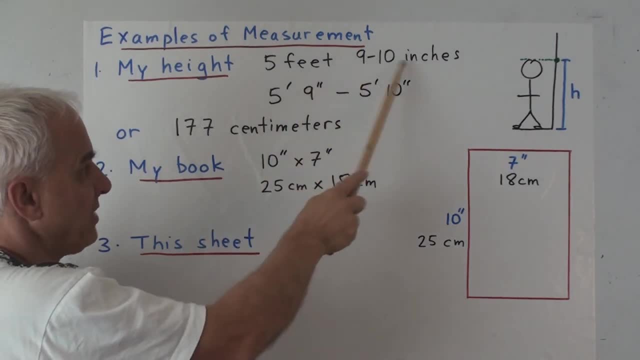 that I made. that's the height H and my height happens to be somewhere between height happens to be somewhere between height happens to be somewhere between 5 feet 9 and 5 feet 10 inches, so I'm 5 feet 9 and 5 feet 10 inches, so I'm. 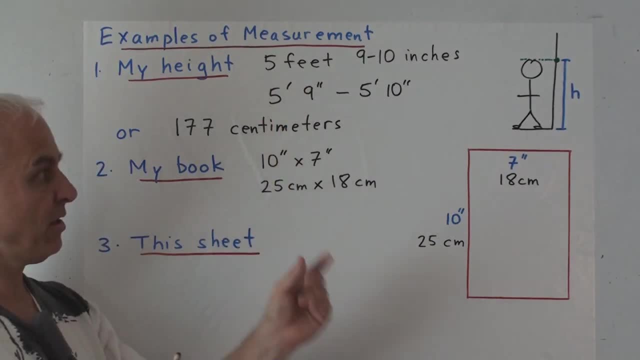 5 feet 9 and 5 feet 10 inches. so I'm using a combination of feet and inches, using a combination of feet and inches, using a combination of feet and inches to measure height, and that's a to measure height and that's a to measure height, and that's a traditional way of doing things. there's 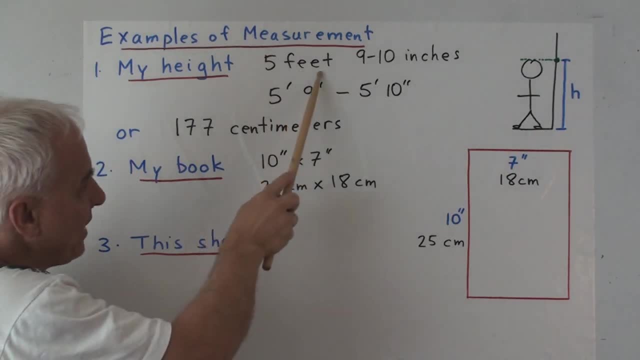 traditional way of doing things. there's traditional way of doing things. there's a notation that's commonly used, so the a notation that's commonly used. so the a notation that's commonly used. so the feet is often represented by a single. feet is often represented by a single. 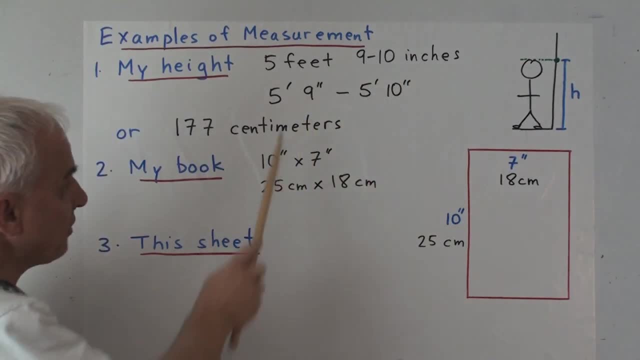 feet is often represented by a single prime and inches by a double prime. so 5 prime and inches by a double prime, so 5 prime and inches by a double prime. so 5 feet 9 inches is represented this way: 5 feet 9 inches is represented this way: 5. 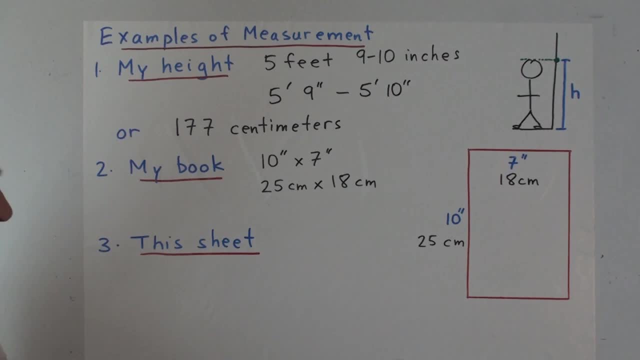 feet 9 inches is represented this way: 5 feet 10 inches represented this way. we feet 10 inches represented this way. we feet 10 inches represented this way. we don't have any fractions yet because don't have any fractions yet, because don't have any fractions yet because we're just doing early K to 6, so far. so 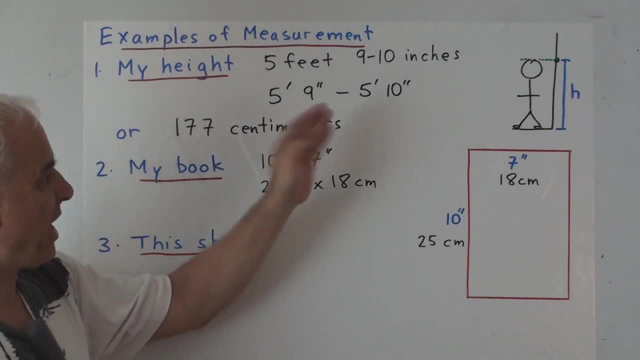 we're just doing early K to 6 so far. so we're just doing early K to 6 so far. so the best we can say is somewhere between. the best we can say is somewhere between. the best we can say is somewhere between 5 foot 9 and 5 foot 10 is my height of. 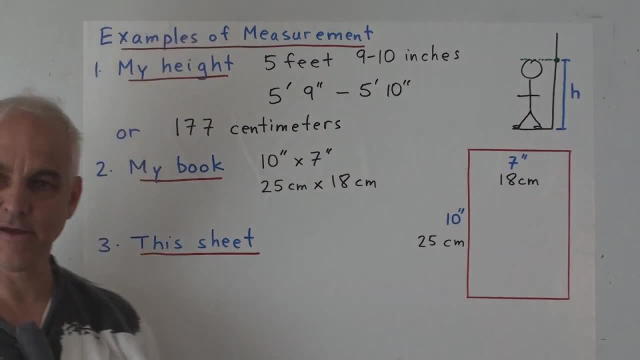 5 foot 9 and 5 foot 10 is my height of 5 foot 9 and 5 foot 10 is my height. of course I could take that mark and then I course I could take that mark, and then I course I could take that mark, and then I could measure that same height in the. 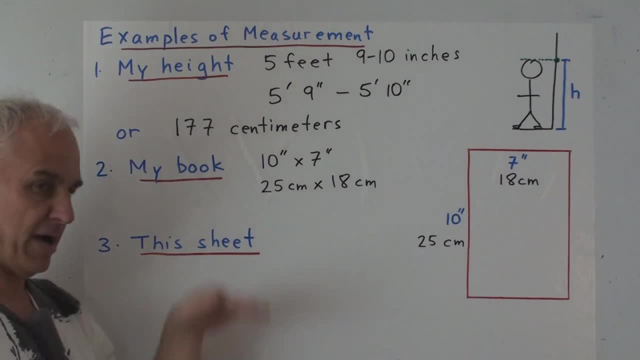 could measure that same height in the, could measure that same height in the metric system. so it would be more than a metric system. so it would be more than a metric system. so it would be more than a meter, but less than 2 meters. so meter, but less than 2 meters so. 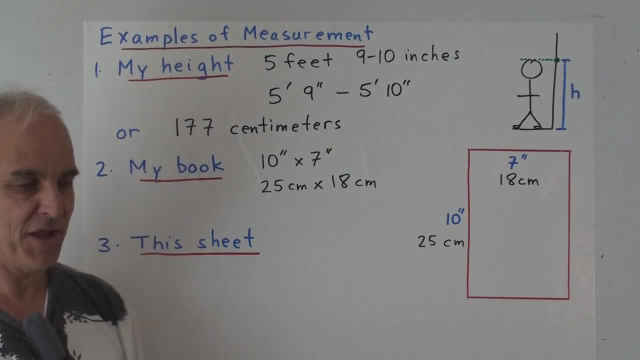 meter but less than 2 meters. so somewhere between 1 meter and 2 meters, somewhere between 1 meter and 2 meters, somewhere between 1 meter and 2 meters is not very instructive, so we want to go. is not very instructive, so we want to go. 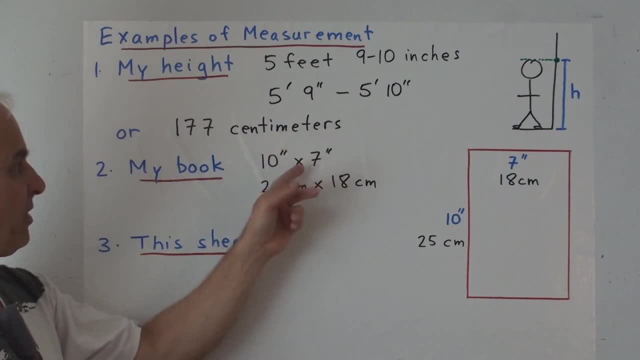 is not very instructive. so we want to go to the finer scale of centimeters and to the finer scale of centimeters and to the finer scale of centimeters and in centimeters. my height is roughly in centimeters. my height is roughly in centimeters. my height is roughly 177 centimeters. so 177 centimeters. 177 centimeters, so 177 centimeters. 177 centimeters, so 177 centimeters. equivalent to somewhere between 5- 9 and equivalent to somewhere between 5- 9 and equivalent to somewhere between 5- 9 and 5- 10 in the imperial system. let's measure. 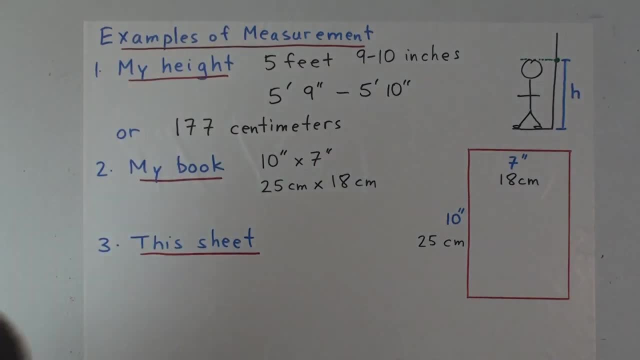 5- 10 in the imperial system. let's measure 5- 10 in the imperial system. let's measure something else. so my book. I've written something else. so my book. I've written something else. so my book. I've written a book and at some point, when you get to, 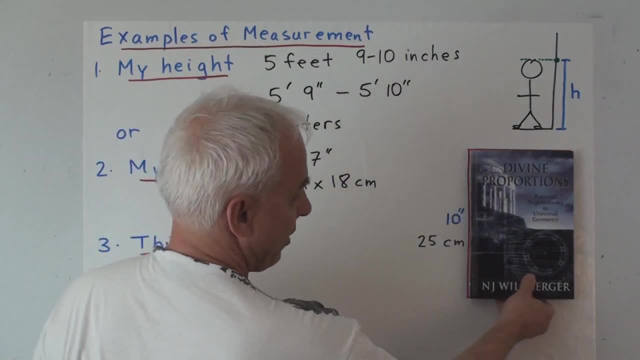 a book and at some point when you get to a book and at some point when you get to high school, you can read my book on high school. you can read my book on high school. you can read my book on trigonometry and there is roughly the 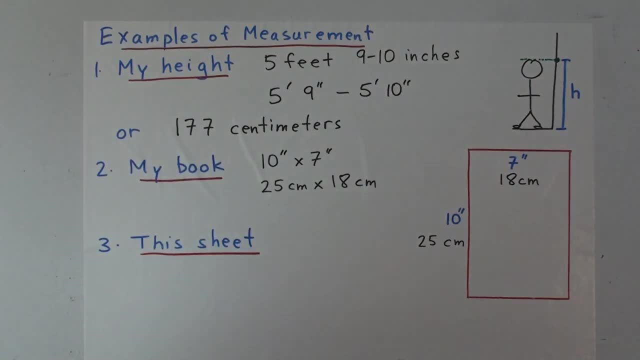 trigonometry and there is roughly the trigonometry and there is roughly the dimensions on my book. so let's measure dimensions on my book. so let's measure dimensions on my book. so let's measure how much that is first of all with an, how much that is first of all with an. 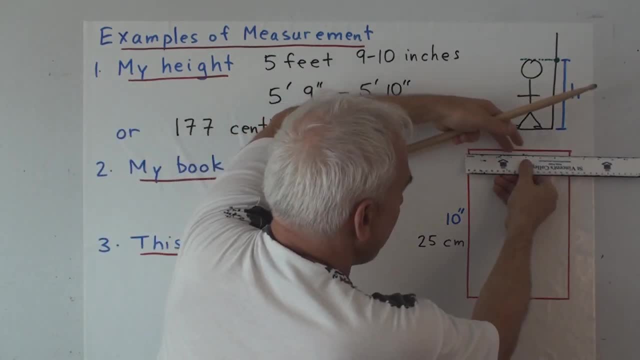 how much that is. first of all with an imperial ruler. so here we have 0, 1, 2, 3 imperial ruler. so here we have 0, 1, 2, 3 imperial ruler. so here we have 0, 1, 2, 3, 4, 5, 6, 7 inches and, in this direction, 0 up. 4, 5, 6, 7 inches and in this direction, 0 up 4, 5, 6, 7 inches and in this direction, 0 up to about 10 inches. we're just going to to about 10 inches, we're just going to. 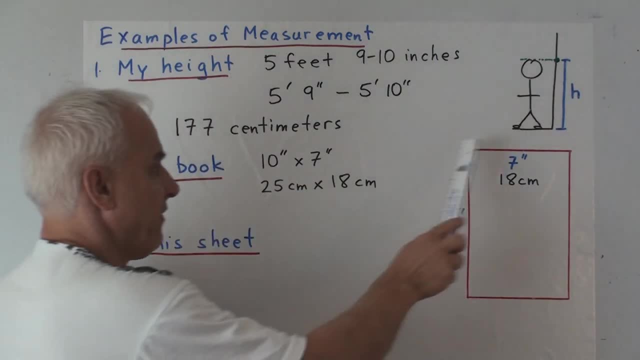 to about 10 inches. we're just going to round to the nearest value. so 7 inches round to the nearest value. so 7 inches round to the nearest value. so 7 inches in that direction, 10 inches high, and in that direction, 10 inches high, and 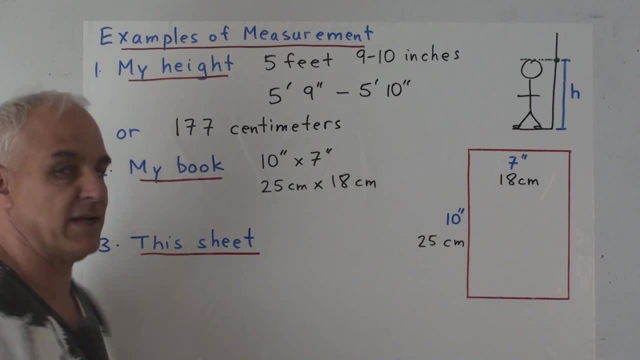 in that direction, 10 inches high, and that rectangle then is a 10 inch by 7. that rectangle then is a 10 inch by 7. that rectangle then is a 10 inch by 7 inch rectangle in the metrical system. inch rectangle in the metrical system. 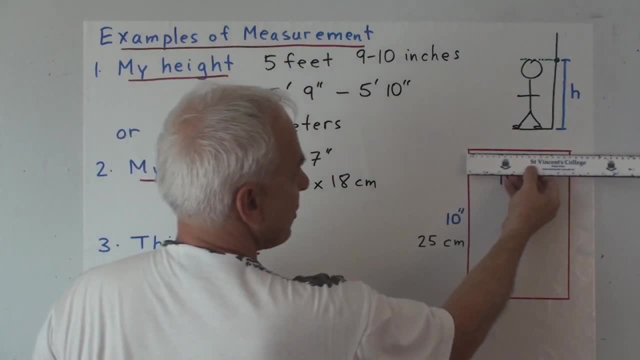 inch rectangle in the metrical system. well, I can flip this thing over there's. well, I can flip this thing over there's. well, I can flip this thing over. there's a metrical scale here, so in centimeters. a metrical scale here, so in centimeters. 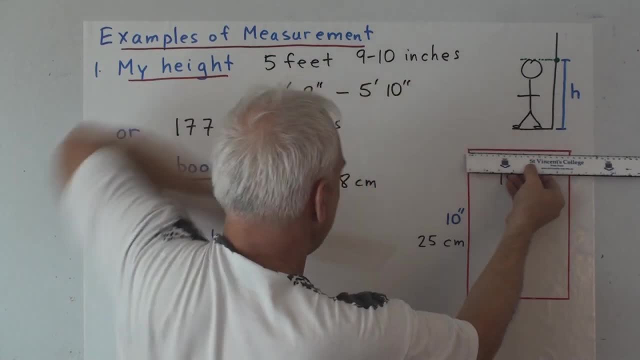 a metrical scale here, so in centimeters, I can read 0 and you won't be able to. I can read 0 and you won't be able to. I can read 0 and you won't be able to read. but it goes up to around 18 there. 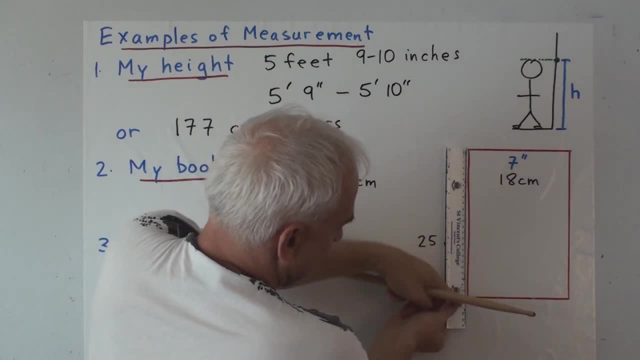 read, but it goes up to around 18 there. read, but it goes up to around 18 there and here: 0 all the way to around 25 a and here: 0 all the way to around 25 a and here: 0 all the way to around 25, a little bit more so this is a 25. 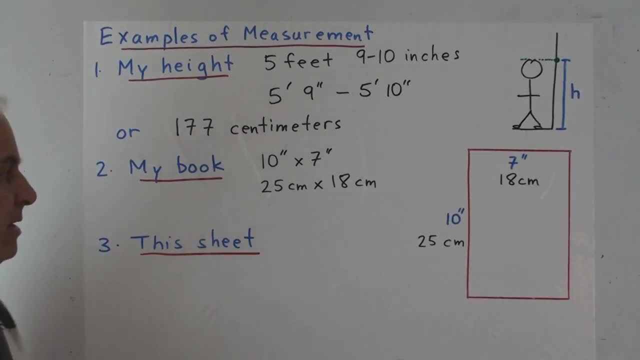 little bit more so this is a 25 little bit more so. this is a 25 centimeters by 18 centimeters in the centimeters, by 18 centimeters in the centimeters, by 18 centimeters in the metrical system. this is the short form. 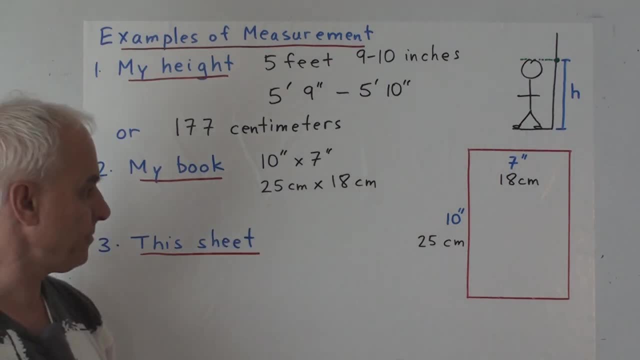 metrical system. this is the short form. metrical system. this is the short form for centimeters- CM. the double prime is for centimeters CM. the double prime is for centimeters CM. the double prime is the short form for inches. let's do one. the short form for inches. let's do one. 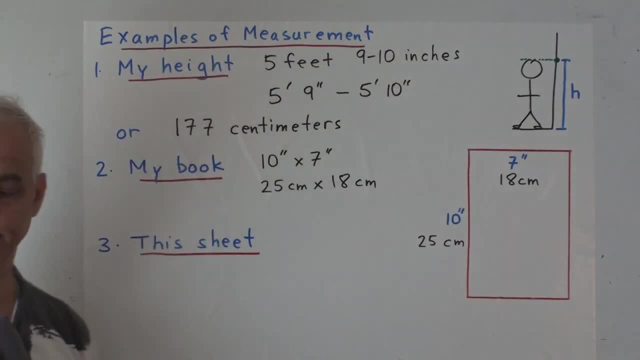 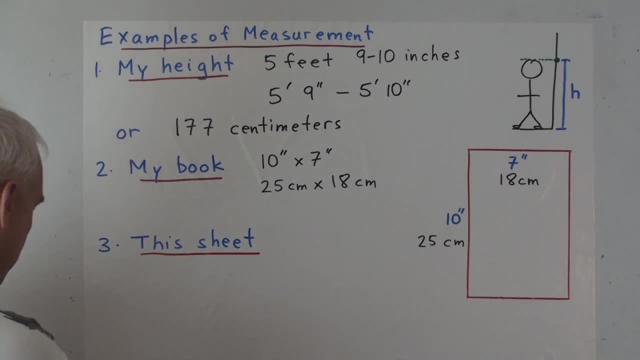 so let's start with the Imperial system. here's my foot and I'm going to measure. here's my foot and I'm going to measure. here's my foot and I'm going to measure this. okay, I'll mark up mark there. that's this. okay, I'll mark up mark there. that's. 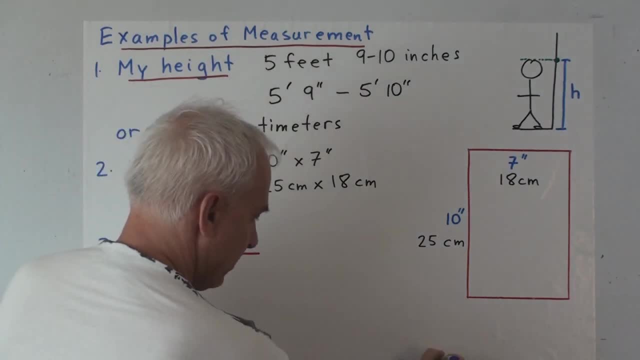 this. okay, I'll mark up mark there. that's one foot and there's another foot and one foot, and there's another foot and one foot and there's another foot, and it's more than a foot. it's about 11. it's more than a foot, it's about 11. 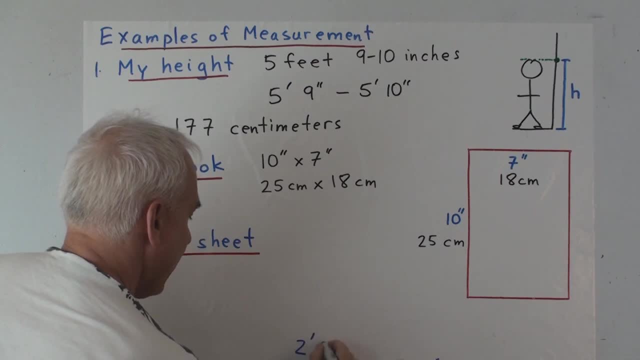 it's more than a foot, it's about 11 inches. say so it looks like we said two inches. say so it looks like we said two inches. say so it looks like we said two feet and 11 inches in that direction. feet and 11 inches in that direction. 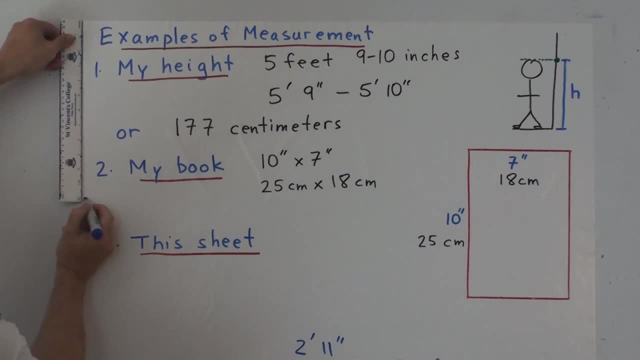 feet and 11 inches in that direction and in this direction and in this direction and in this direction: zero lines up to 12. there's one foot, zero lines up to 12. there's one foot, zero lines up to 12. there's one foot there and it's 11 and a half. let's say: 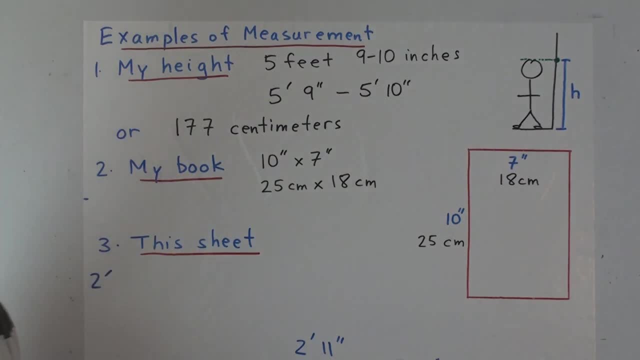 there, and it's 11 and a half, let's say there, and it's 11 and a half, let's say two feet, so two feet in that direction. two feet, so two feet in that direction. two feet, so two feet in that direction. and now, in the metrical system, I take my 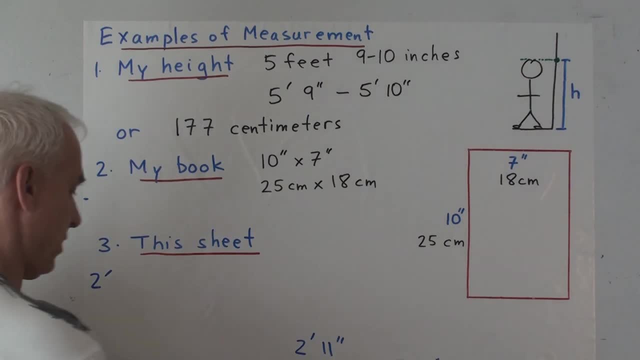 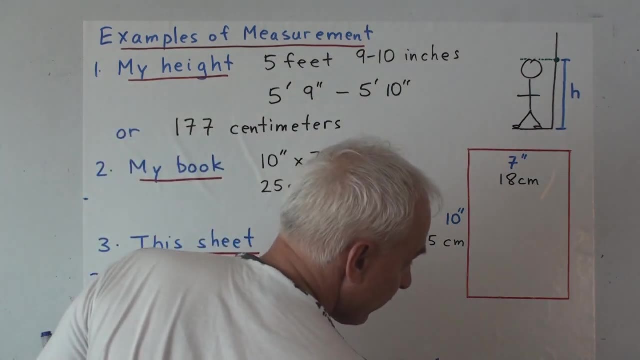 and now in the metrical system I take my. and now in the metrical system I take my metrical ruler. here it is, and we go metrical ruler, here it is, and we go metrical ruler, here it is, and we go from here to here and it's showing okay. 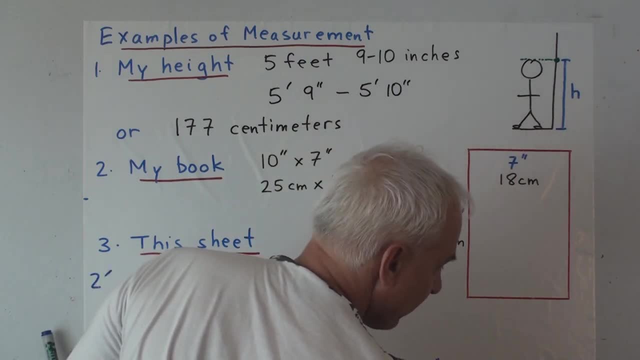 from here to here, and it's showing okay. from here to here, and it's showing okay. eight hundred and fifty eight, sixty. eight hundred and fifty eight, sixty, eight hundred and fifty eight, sixty eight, seventy eight, eighty, it's about 88. eight seventy eight, eighty, it's about 88. 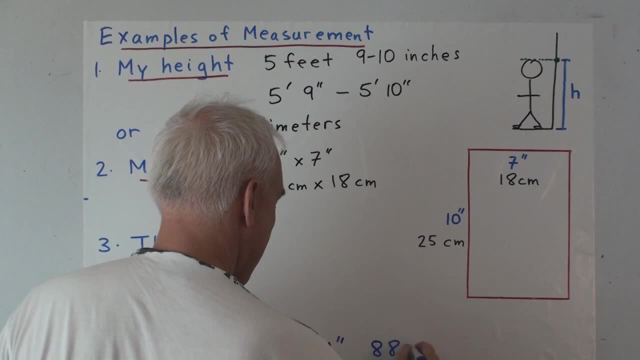 eight, seventy, eight, eighty. it's about 88 centimeters. remember: 100 centimeters is centimeters. remember 100 centimeters is centimeters. remember 100 centimeters is all the way and this is 88 centimeters, all the way and this is 88 centimeters. 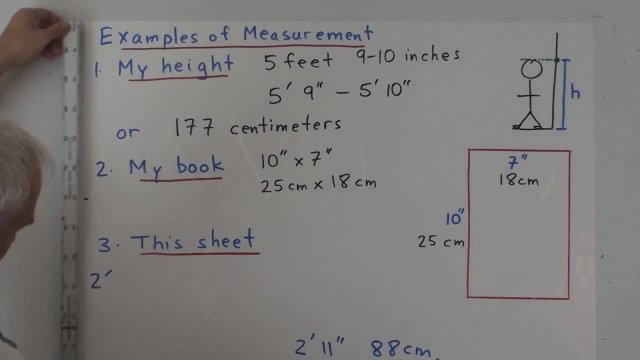 all the way, and this is 88 centimeters, and in this direction about 600, and in this direction about 600 and in this direction about 600 millimeters or 60 centimeters in that millimeters or 60 centimeters in that millimeters or 60 centimeters in that direction. so in the imperial system we 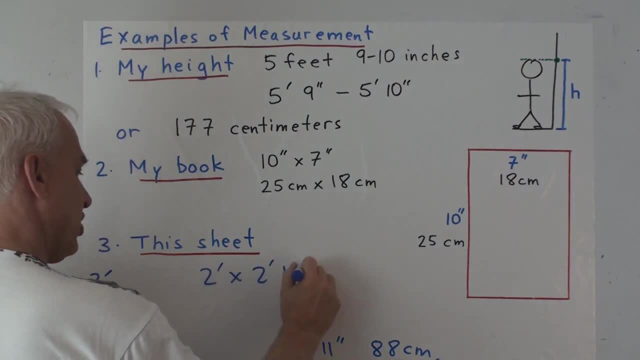 direction. so in the imperial system we direction. so in the imperial system we would say it's two feet by two feet 11 would say it's two feet by two feet, 11 would say it's two feet by two feet 11 inches, inches, inches, and in the electrical system it's 60. 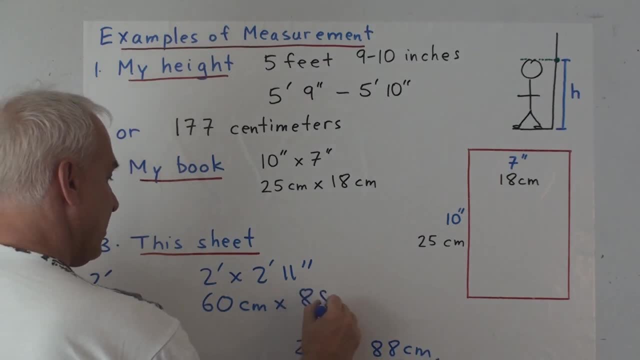 and in the electrical system it's 60, and in the electrical system it's 60 centimeters by 88 centimeters, and when centimeters by 88 centimeters, and when centimeters by 88 centimeters, and when we're measuring things, we have to get. 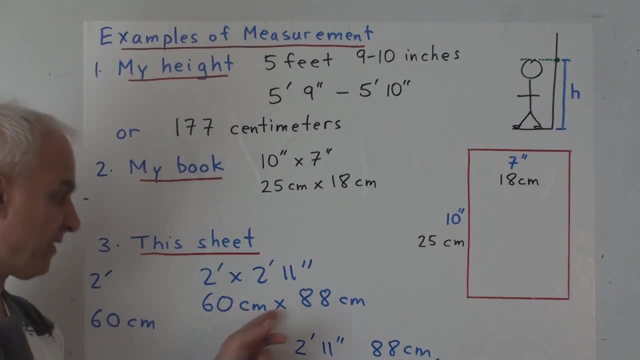 we're measuring things we have to get. we're measuring things we have to get used to actually specifying the units. so used to actually specifying the units. so used to actually specifying the units. so including the centimeters, or including including the centimeters, or including including the centimeters, or including the markings for feet and inches, that's. 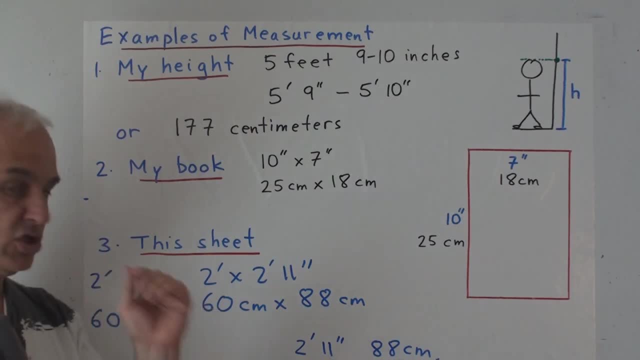 the markings for feet and inches. that's the markings for feet and inches. that's an important part of the measurement, is an important part of the measurement is an important part of the measurement is to identify which units we are using. to identify which units we are using. 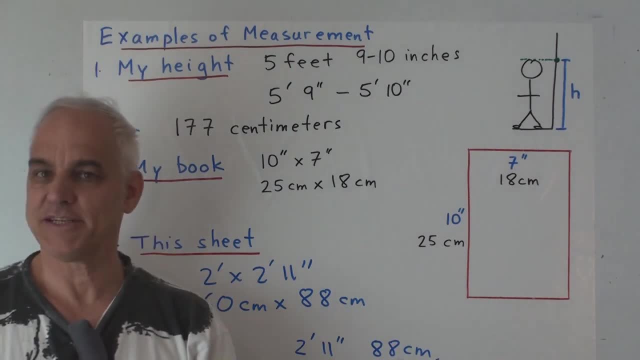 to identify which units we are using. alright, so that's good. we've talked. alright, so that's good, we've talked. alright, so that's good. we've talked about length. obviously the next thing to about length, obviously the next thing to about length. obviously, the next thing to talk about is weight, right, so next time. 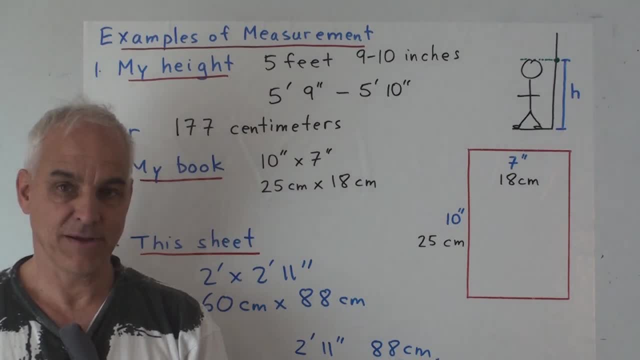 talk about is weight right. so next time, talk about is weight right? so next time we'll have a look at weight measuring. we'll have a look at weight measuring. we'll have a look at weight measuring- weight both in the metrical and in the weight, both in the metrical and in the. 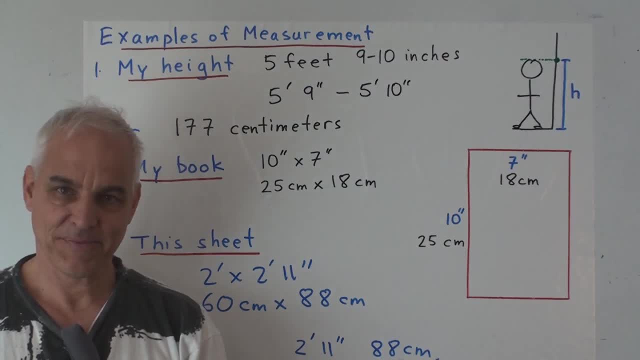 weight, both in the metrical and in the imperial system. I hope you'll join me for imperial system. I hope you'll join me for imperial system. I hope you'll join me for that. I'm Norman Wahlberger. thanks for that. I'm Norman Wahlberger, thanks for. that I'm Norman Wahlberger. thanks for listening.